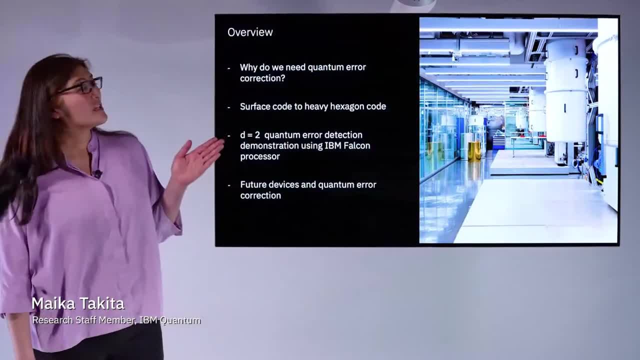 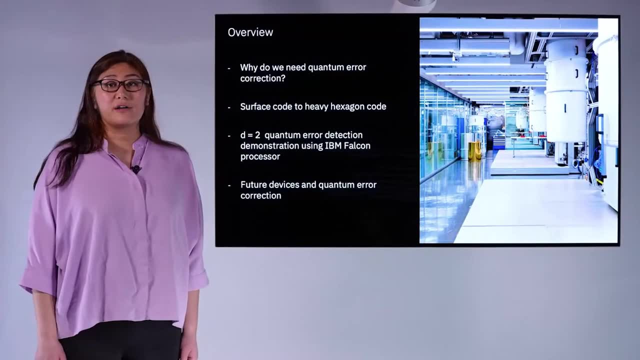 error correction more practical. So here's an overview of my talk. First, why do we need quantum error correction? Quantum systems are inherently noisy and we need a way to deal with these noises. The way classical computers also use some type of error correction. I'll discuss some similarities. 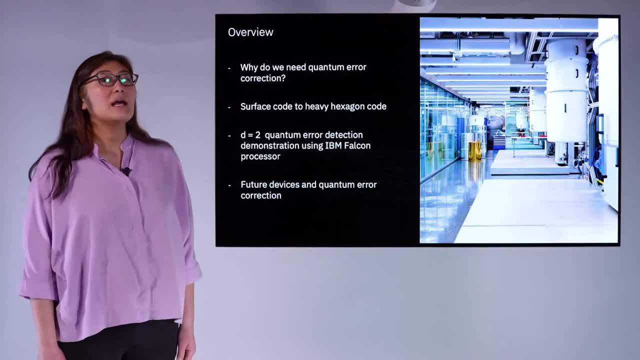 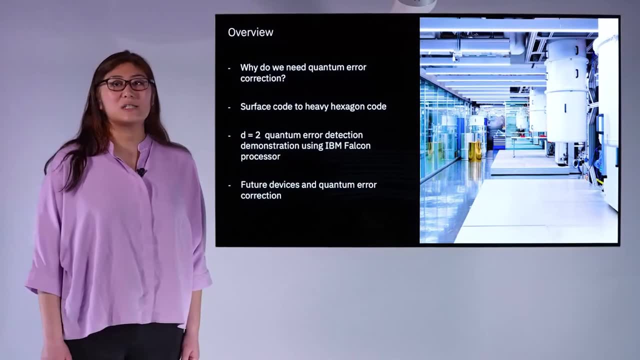 and differences when working with quantum systems. I will then introduce you to a popular quantum error correction code, a surface code that is ideal for near-term to realize with current hardware technology, and tell you more on the innovations IBM has made in co-designing. 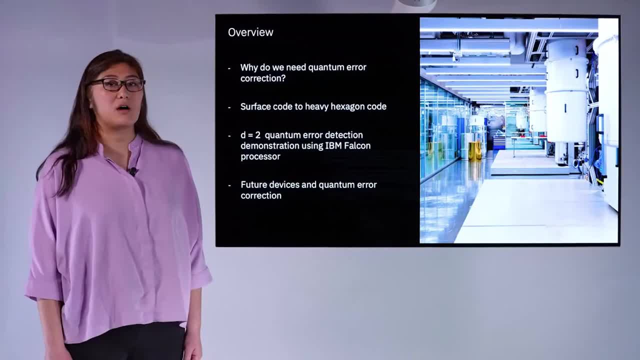 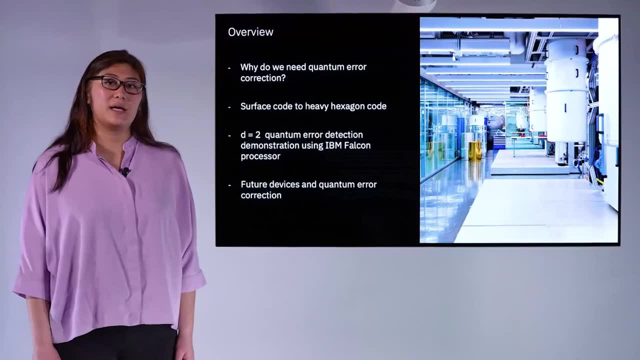 new heavy-hexagon code that is more practical. Thank you. The main focus of this talk will be on the progress we have made in superconducting qubits at IBM and recent demonstration of the D equals 2 error detection code that we have done using. 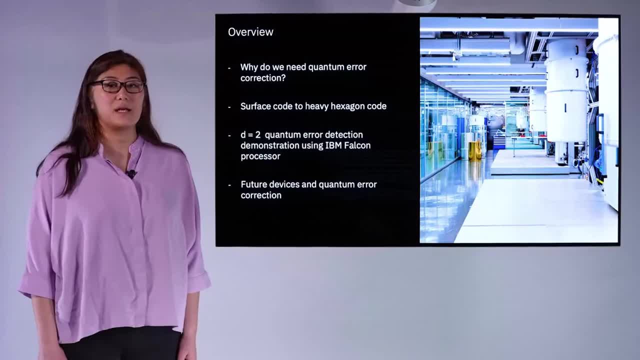 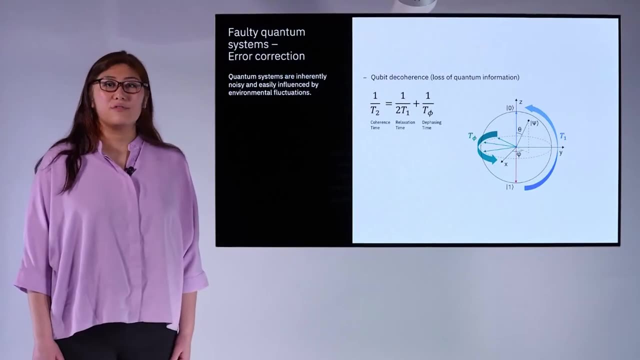 one of IBM's 27-qubit Falcon processor. Finally, to wrap up the talk, I'd like to discuss how IBM quantum hardware roadmap aligns with future work on quantum error correction. Faulty quantum systems require some type of error correction. But first, what do I mean by faulty? 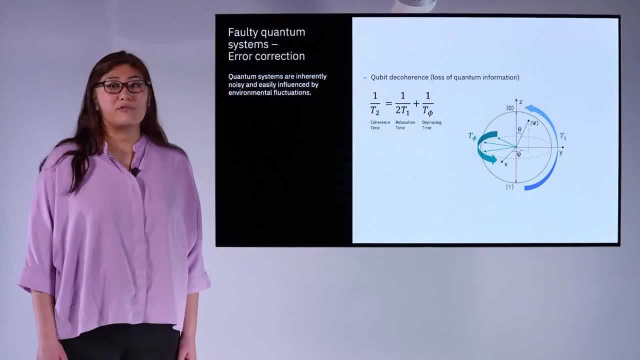 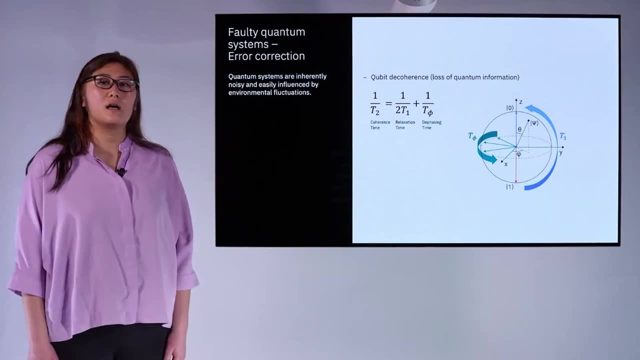 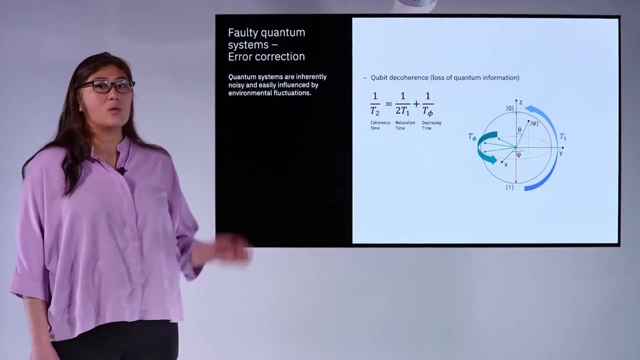 Quantum systems are inherently noisy and easily influenced by environmental fluctuation. Some typical errors in quantum systems are qubit decoherence, which is a loss of quantum information. So here is a block sphere representing single qubit, with zero state on the north pole, and 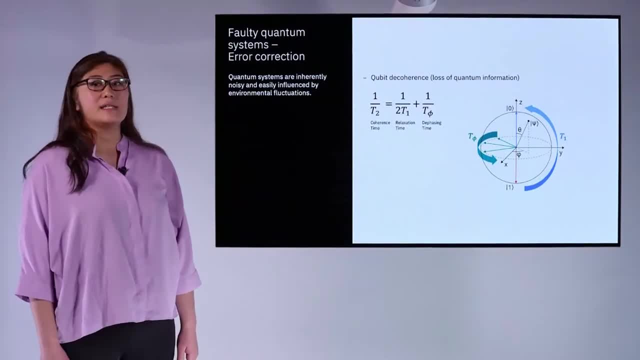 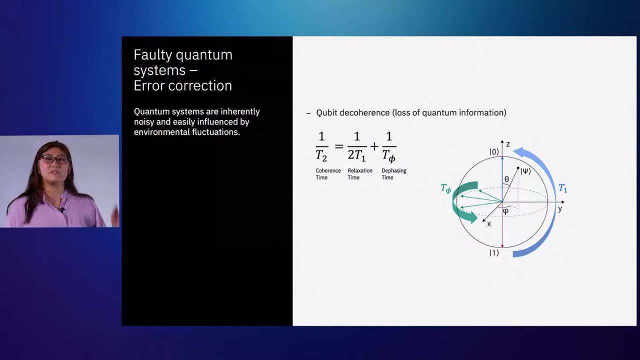 one in the south pole, T1, relaxation time is decay from one to zero state. as you see here in a big blue arrow, Qubits not only have zero and one state but can also be in a superposition state where phase of the state also carry information. 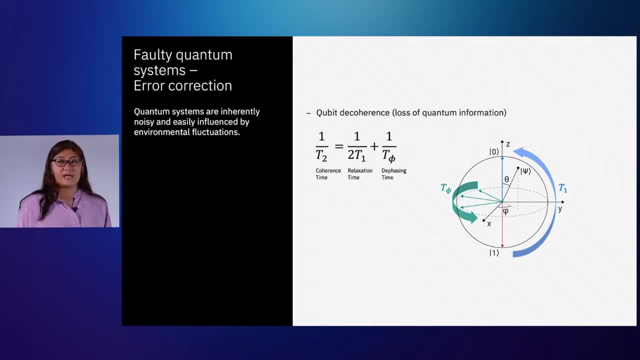 T5 defacing time is randomization of the phase phi, as you see here in green arrow, And these two- T1 and T5, contribute to T2 coherence times. Both T1 relaxation time and T2 coherence times have improved over the years, As you may have. 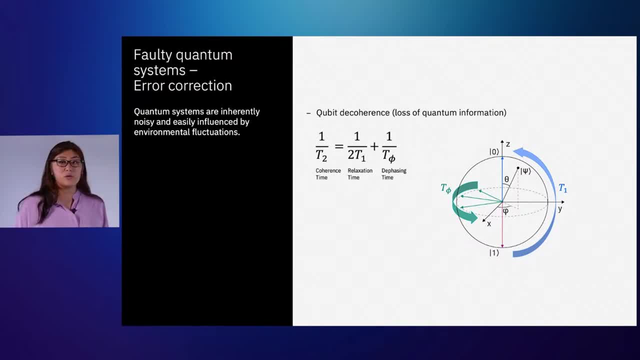 heard how recently we have reached average of about 300 microsecond T1 and T2 on a large 27-qubit Falcon processor. Nonetheless, this is still a large source of error in our systems. Other errors in the systems are gate errors that could come from poor calibration state. 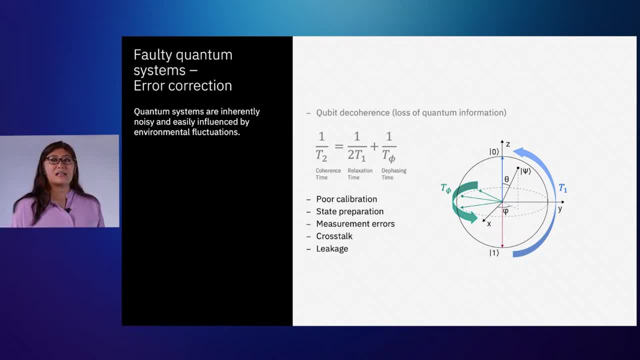 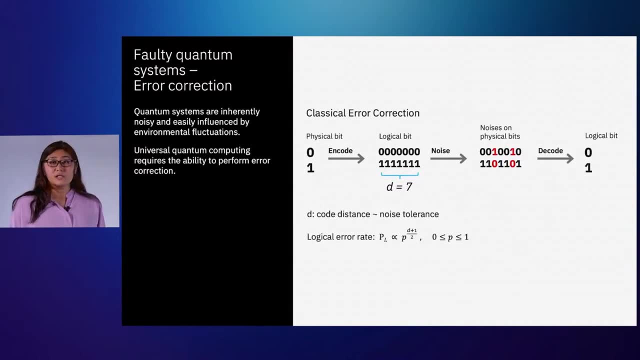 preparation and measurement errors, crosstalk errors and leakage errors- that takes your qubit out of the computational basis, to name a few. However, quantum systems are faulty and to build a universal quantum computer to solve large and complex problems we will need some type of quantum error correction. 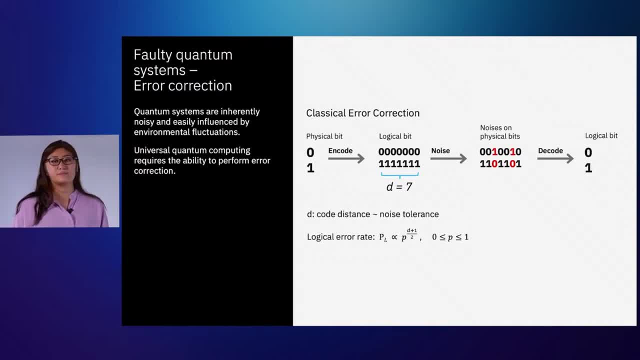 So let's start from reviewing how classical error correction works. In a classical system, each physical bit can be encoded into many zeroes and ones. When there is some noise, some of the bits can flip from zero to one and one to zero. In this example, the third and sixth bits in red have flipped. 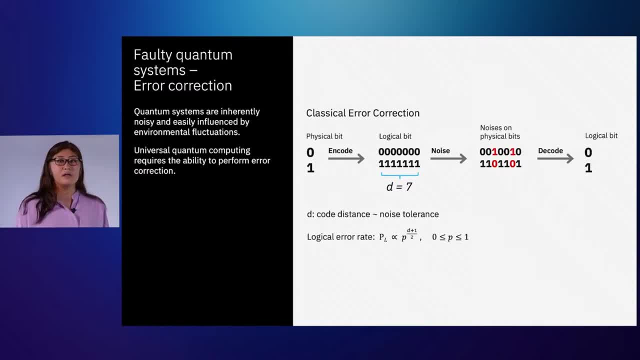 But as long as less than half of the copies experience a bit flip, you can look at the bit string and simply do a majority vote to decode back into the correct state. Here the code distance D roughly indicates the amount of noise tolerance and, as you, 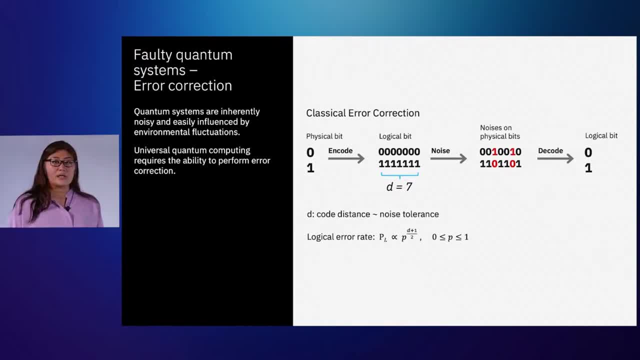 see here you can expect a lower logical error PL as you increase the distance D, with some error rate P, which is between 0 to 1.. So that was classical error correction. now, how about quantum error correction? Can we do the same? 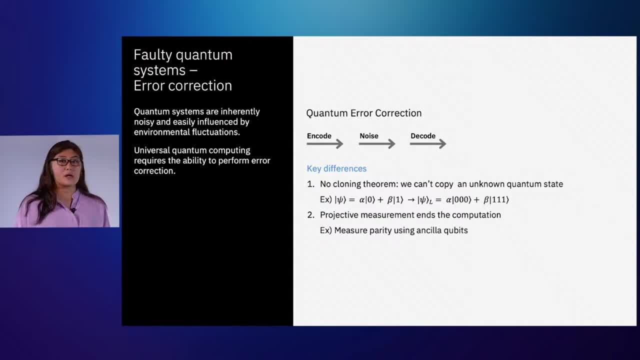 Similar to classical error correction. quantum error correction relies on encoding- dealing with some noise and decoding, But key differences are that we can't copy an unknown quantum state, as proved in no-cloning theorem, But as you see in this example. 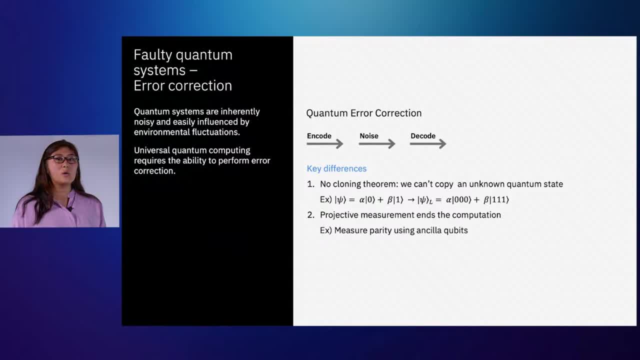 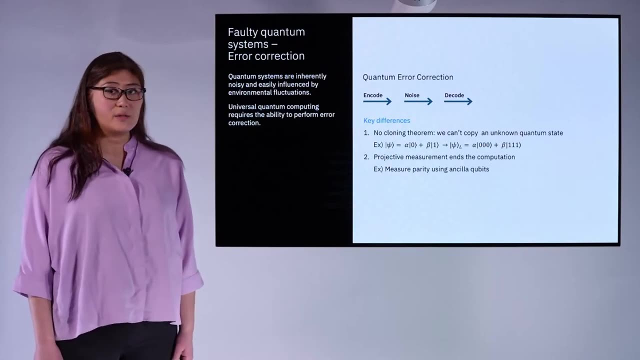 rather than making a copy of psi, you can encode psi logical into a state like 000 plus 111 and use that as your logical qubit. Another difference is that when you measure a qubit it can destroy entanglement and end the computation. 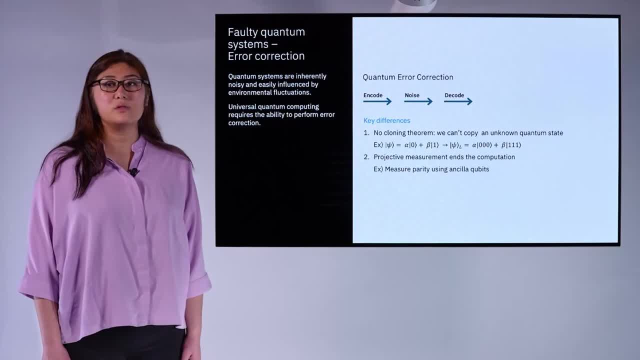 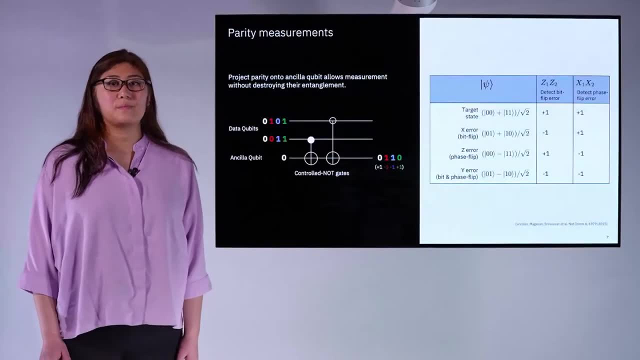 So to get around this, we can use another ancilla qubit that we use to measure a parity of data qubits. So let's talk a bit more about parity measurement. next, The circuit shown here in the left of the slide is the sample circuit that will provide. 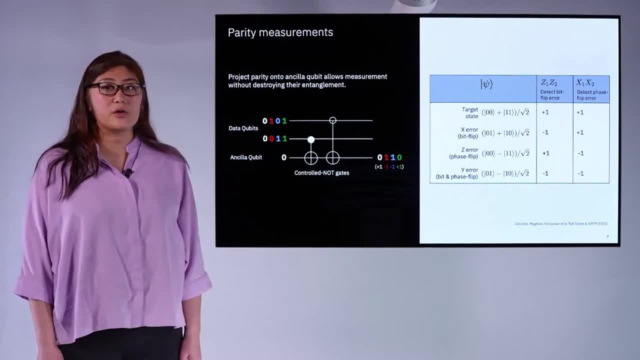 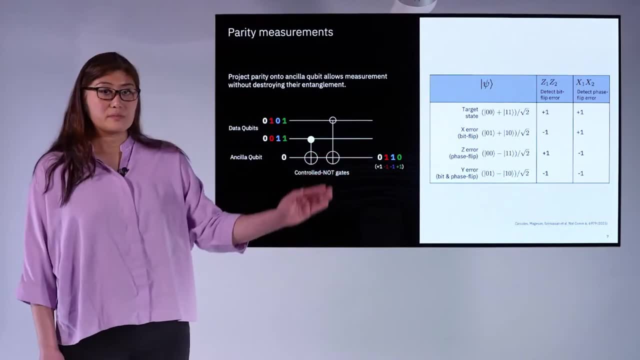 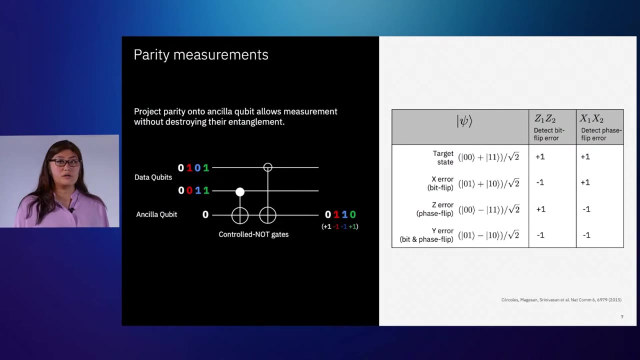 a parity of the two qubits using a third ancilla qubit, And the left plot is to illustrate what parity measurements are, And the right table is an example where we can use the parity to detect errors. Parity of the bit string could be even or odd, and we can find this by measuring the. 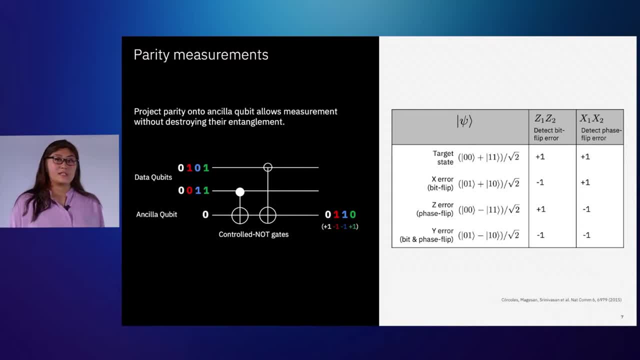 ZZ operator. ZZ parity is a very common error in quantum computing. ZZ parity measurements can have either plus one or minus one eigenvalues, which corresponds to even or odd parity. In this circuit, measuring zero on the ancilla qubit corresponds to plus one eigenvalue or 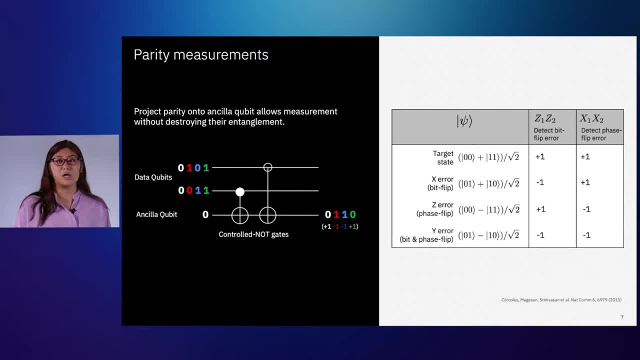 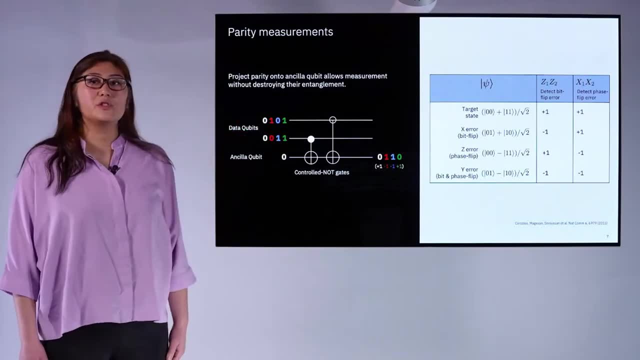 even state and measuring one corresponds to minus one eigenvalue or odd state. If you follow the colors here, the white and the green inputs show 0, 0, and 1, 1,, which have even parities. 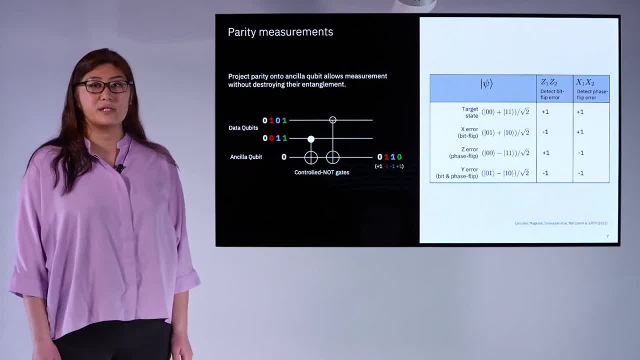 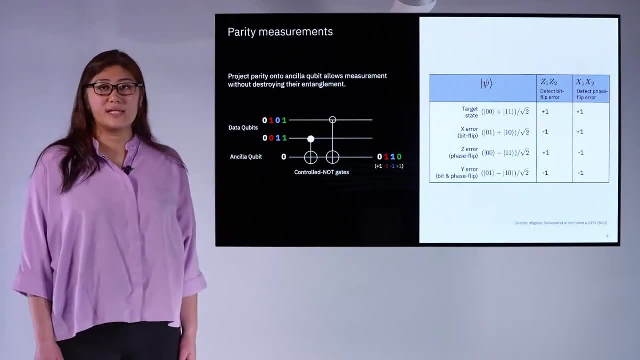 If you measure the third ancilla qubit and probe using the third ancilla qubit, what you measure is 0, that tells you that it has an even parity. The red and the blue states have odd parities which are confirmed when running. 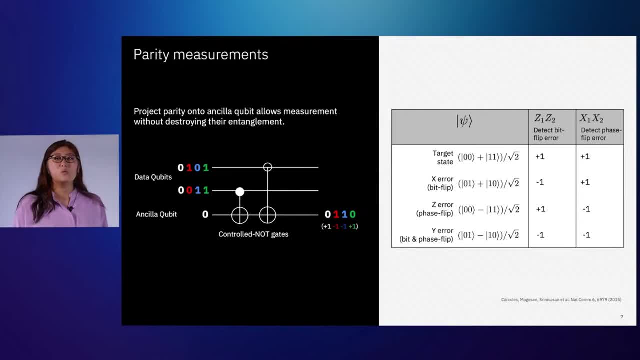 through this circuit that leads to an ancilla qubit being 1, which corresponds to negative eigenvalue. Using the circuit by projecting parity onto the third ancilla qubit, it allows you to measure the parity of the input qubits without destroying the entanglement. 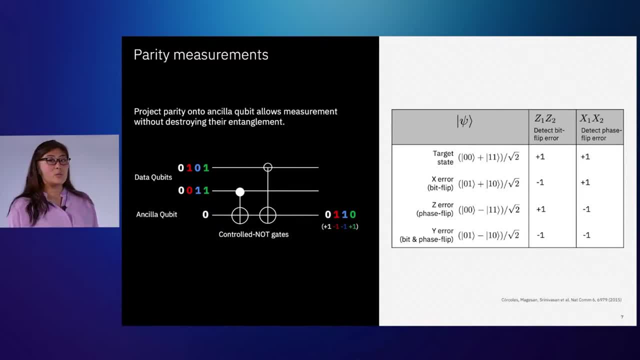 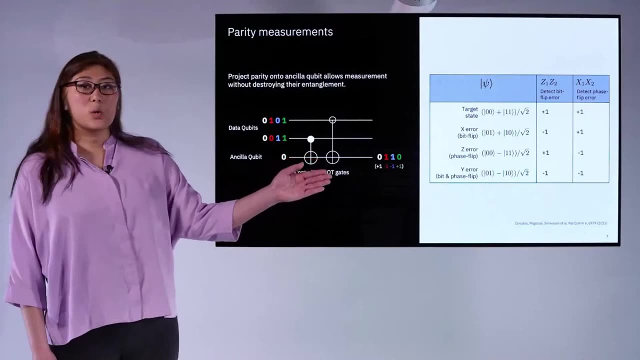 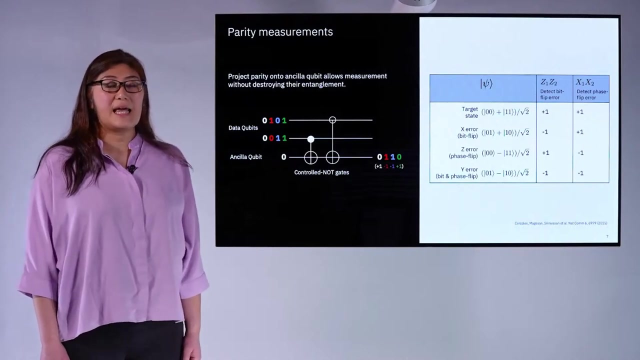 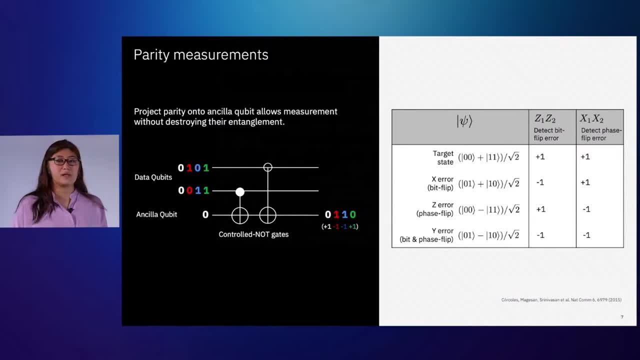 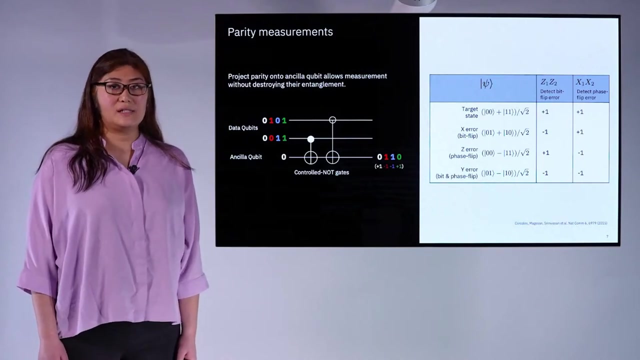 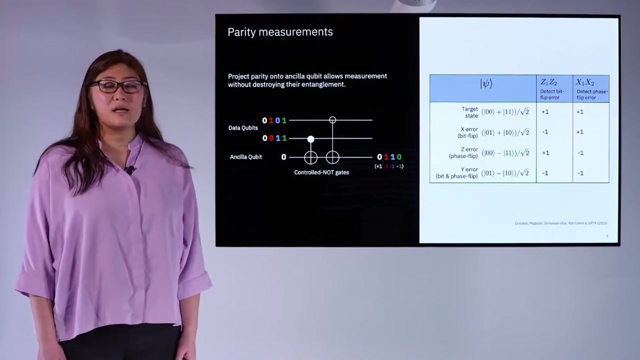 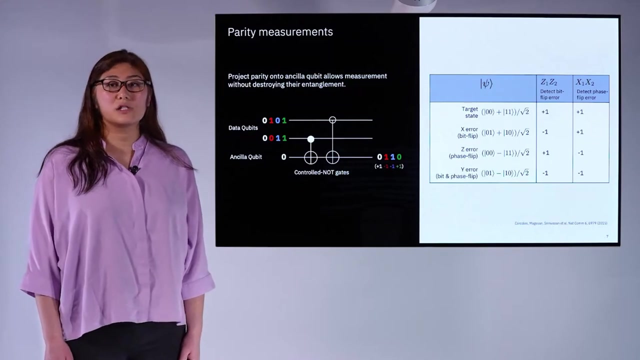 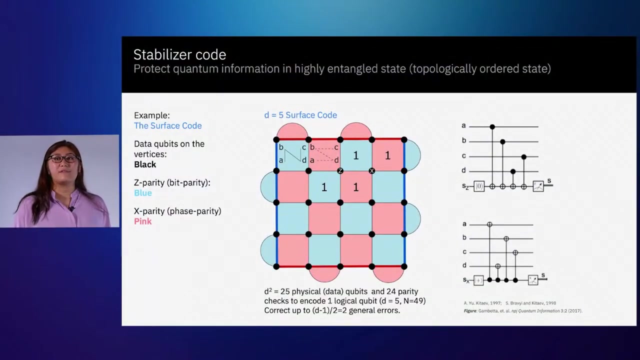 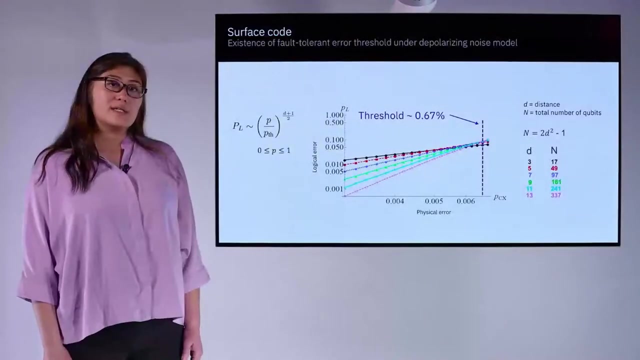 One of the appeals of working with surface code is that it has a relatively high threshold. So what does that mean? Here I have a simulation plot. 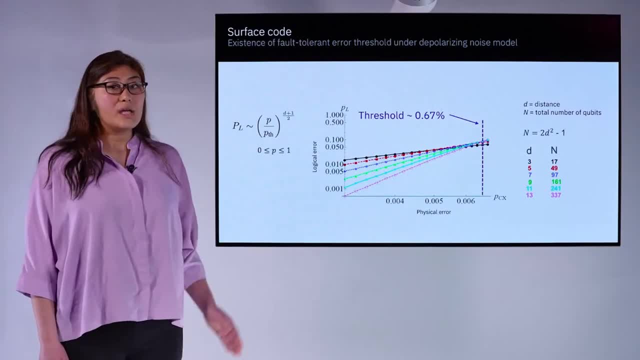 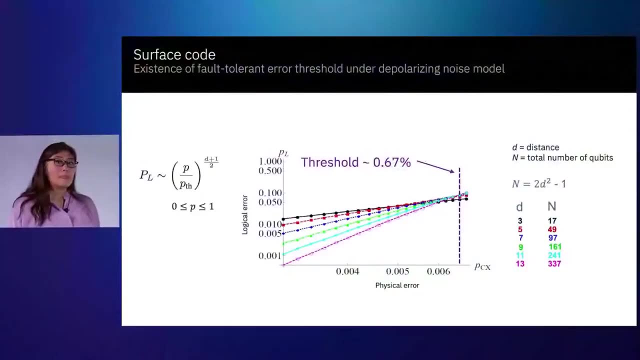 of logical error at different distances. While you sweep the error of this physical qubit, you use to encode a logical qubit. So let's focus on the 2 curves: The black, where it has smallest number of qubits with smallest distance, distance 3. and the magenta curve, with more qubits, with distance 13.. So when the physical 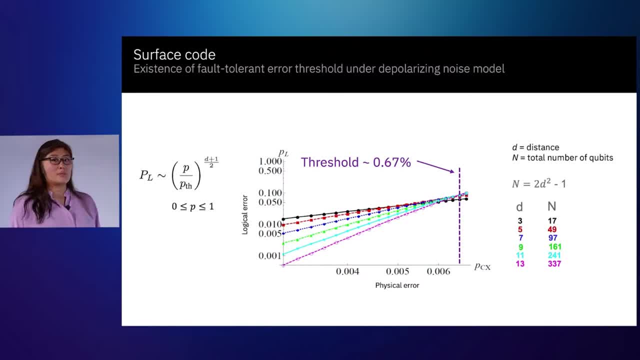 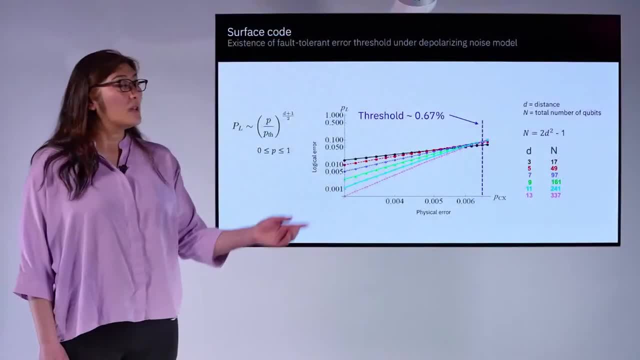 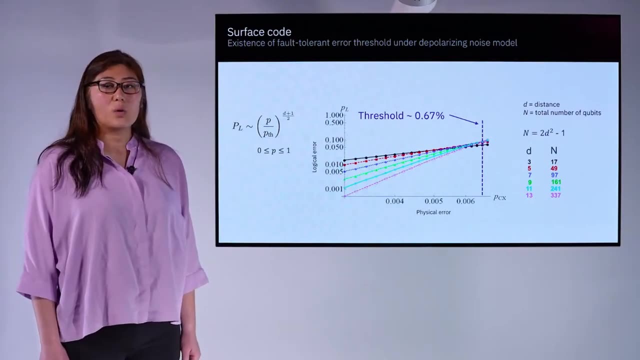 error is high above the threshold where it's shown in purple line, the larger the distance with more qubits result in higher logical error. But below this purple line at the low physical error, as you increase the distance you can get lower and lower logical error. 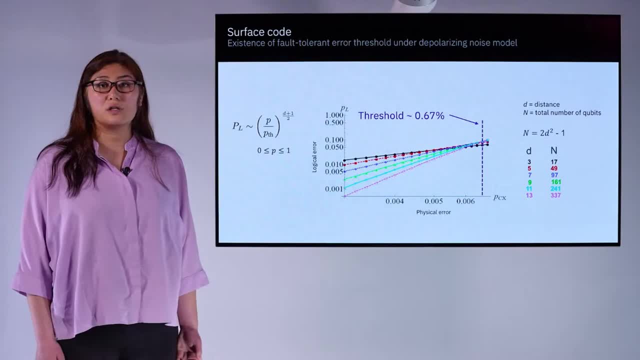 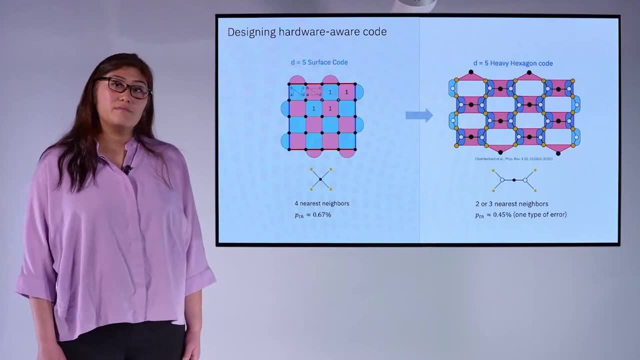 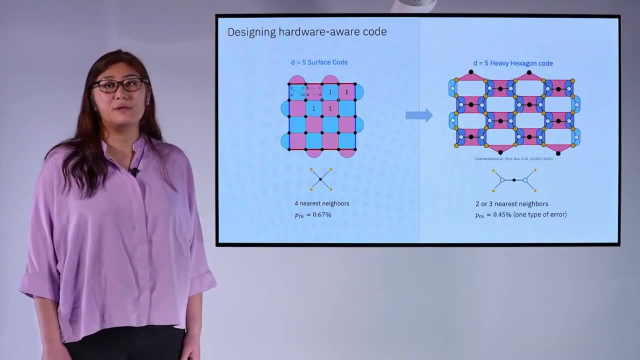 So you see the benefit in using more qubits to encode a logical qubit. if you have low enough physical errors, The surface code is an attractive choice, especially for the superconducting qubits community due to these properties, which is the reason IBM had followed the path in building. 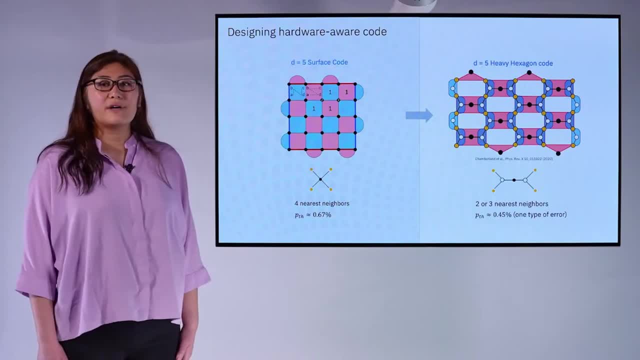 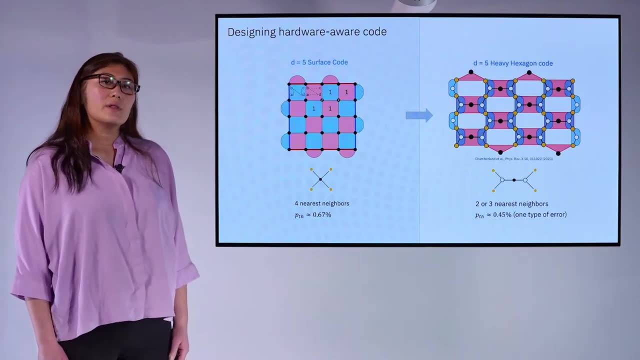 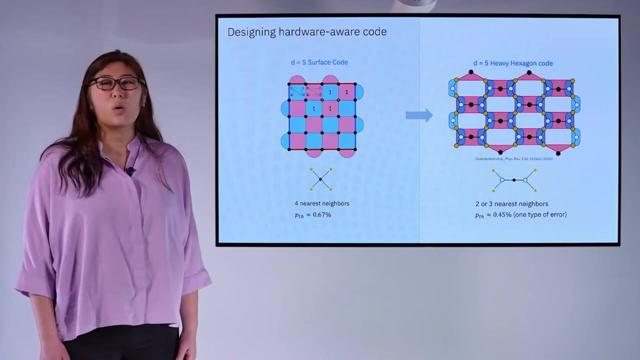 this lattice in the past, Although what we had found was that the surface code requiring four nearest neighbors to run the parity checks are difficult to make. So the main difficulties come from one frequency: crowding that leads to collisions that make it harder, or even 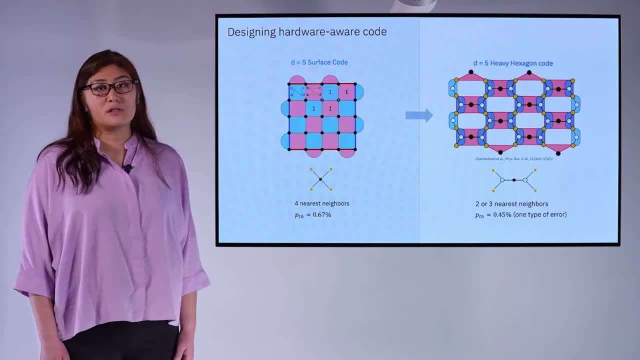 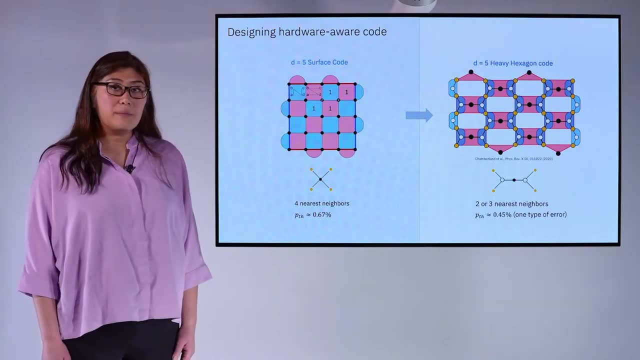 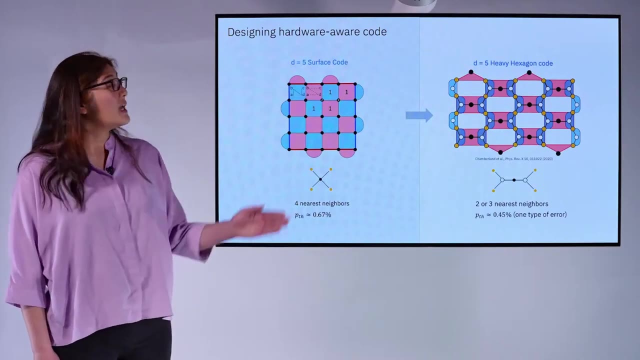 impossible to tune up gates and two crosstalk because there are so many qubits coupled to each one. So IBM has been developing larger and larger superconducting qubits system in the recent years. but we have modified the connectivity so that it is in a heavy hexagon lattice And in this lattice there are at most three. 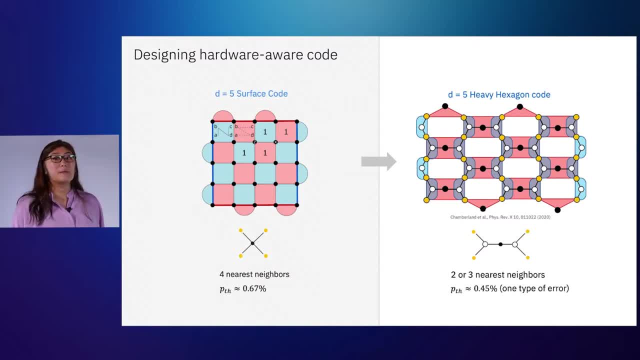 nearest neighbors on each qubits And a lot of them- the black and the orange qubits in this picture- only have two nearest neighbors. This change in qubit layout increases the yield of fabricating a collision-free device. So now we don't have the nice square lattice that you can map surface code to, but the 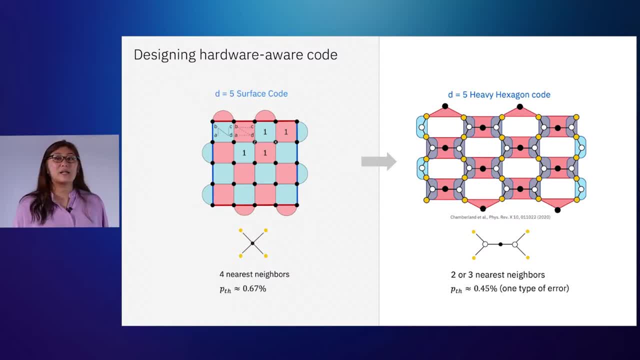 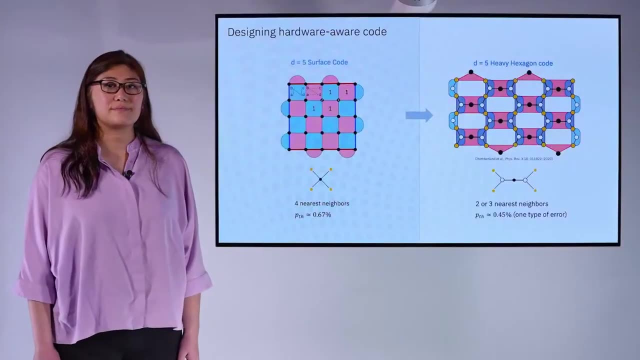 theorist from IBM came up with a new hybrid code called the heavy hexagon code, that you can encode logical qubits similarly to how it was done in surface code, And the threshold for one type of error is around 0.45%, which is not much lower than the surface code. 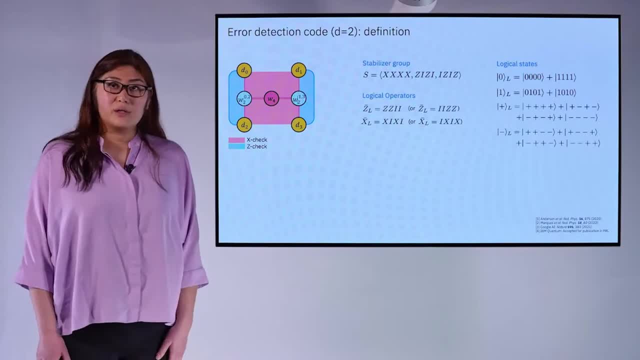 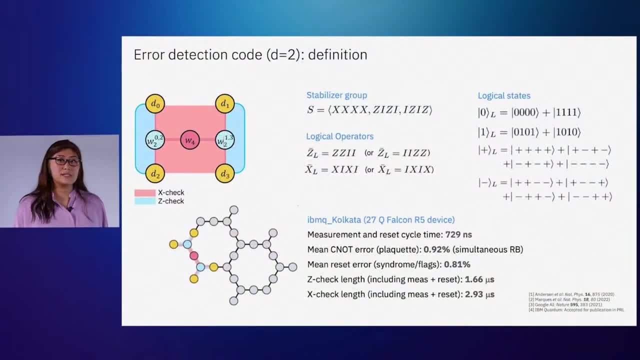 This example code is called the 4-word code. This example code is called the 4-word code. In this example code we Grace is gonna punctualize 4 into 4, so소� integer shows that 1 and R are. 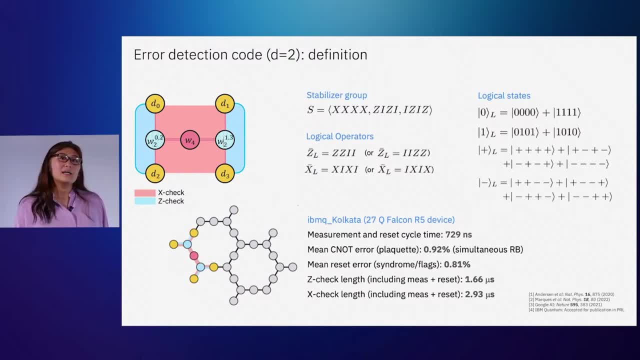 3 Promise In this codeuuuu kan term. Similar color scheme as before pink square denotes that the four orange data qubits in its corner are checked for their phase parities using the pink ancilla qubits, and these two blue qubits are also used as flat qubits for phase parity checks. 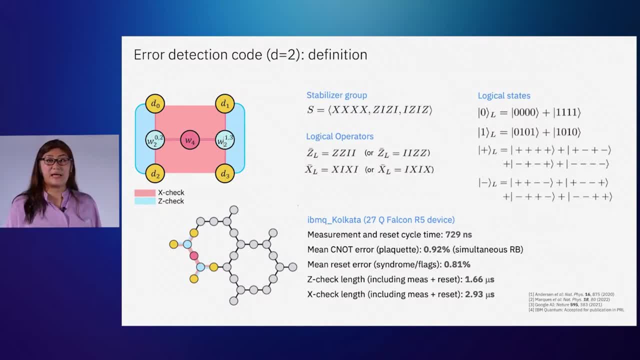 Blue rectangles: check for the bit parity using the blue qubits, again this time as Z parity ancilla qubits. This code can be mapped onto a section of IBM's 27 qubit Falcon processor, and the parity checks or the stabilizers that we will measure, are weight 4 X checks and 2 weight 2 Z checks. 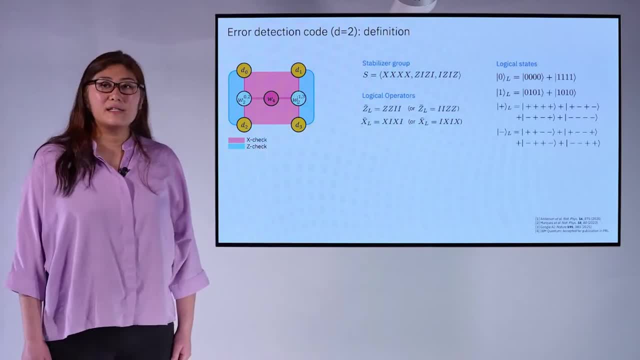 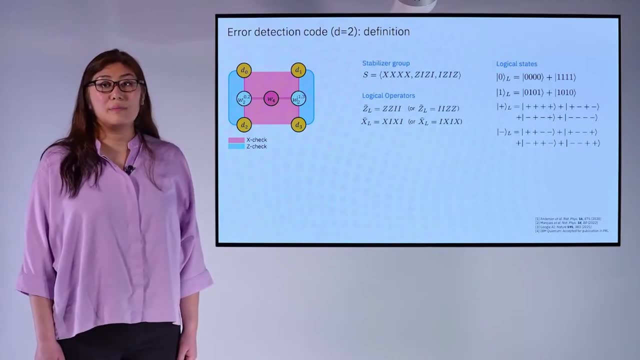 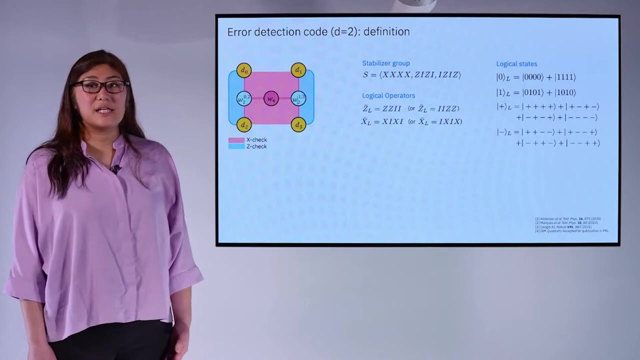 Logical gates and states are defined here and you can apply these logical gates to the state to the right And in the surface code example I mentioned how we repeat the parity checks over and over to keep detecting errors. To do this, we need to keep measuring and reusing the ancilla qubits as you run more. 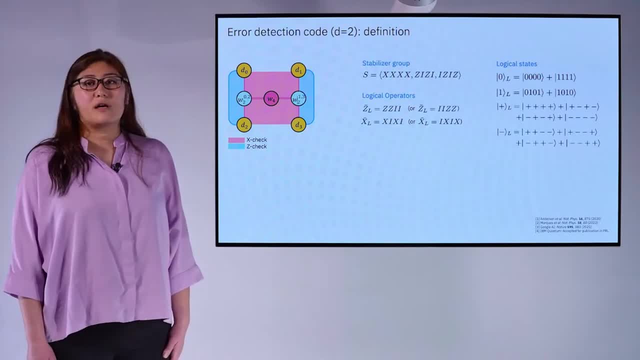 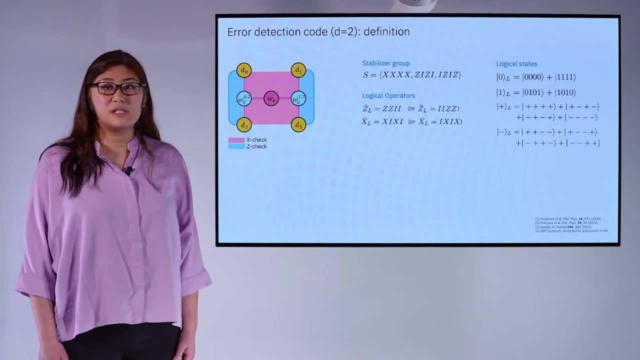 and more parity checks. Ancilla qubits are initialized each time after the measurements and this is done by applying a conditional reset using FPGA to determine the state of the qubit and apply a bit flip depending on the outcome of the measurement. This is a very difficult task when trying to run very fast in similar times as what? 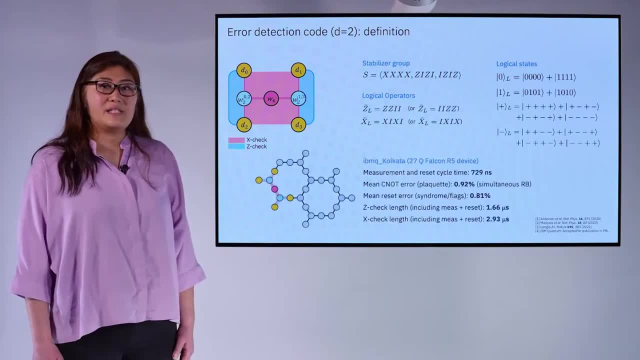 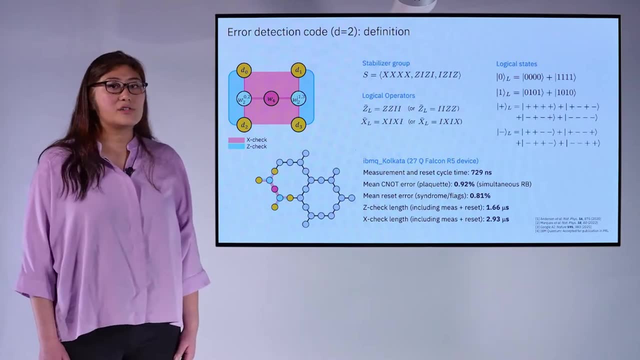 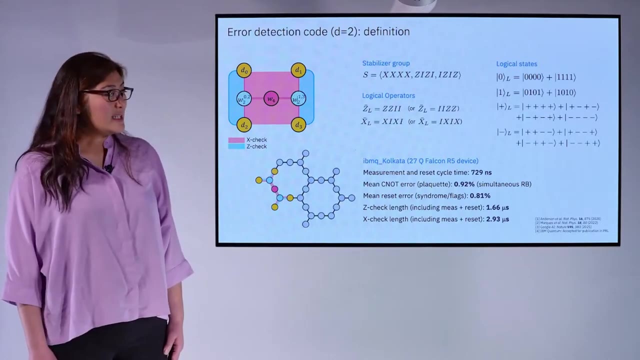 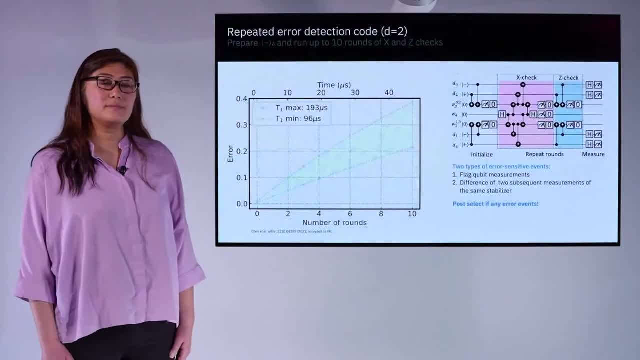 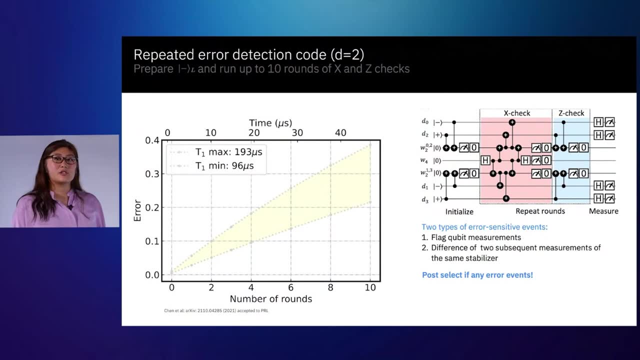 And the time being onion down which causes error to occur is around 1.7 microsecond and X checks takes about 2.9 microsecond. In this slide you'll see an error plot against time or rounds, and rounds are defined in. 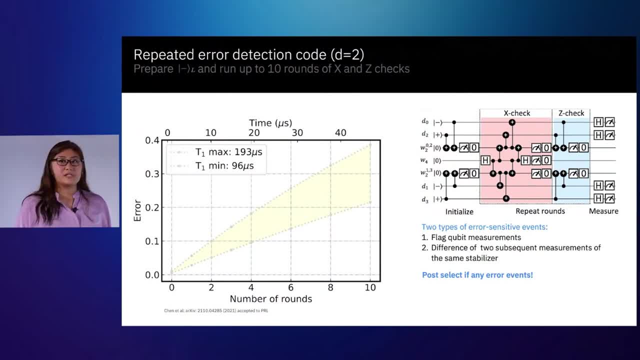 the circuit drawn in the right, where one pink region and one blue corresponds to one round of error detection. So earlier in the talk I discussed several errors that can be present on the quantum system. Here, to compare how well we can preserve Rn, bef and Rf result, let's first look at the result. let's first consider error that arises from T1 relaxation time. A qubit, when prepared in one state, decays to zero state with average lifetime T1, and 7 qubits we used for this experiment has T1 times ranging from 96 to 193 microseconds. 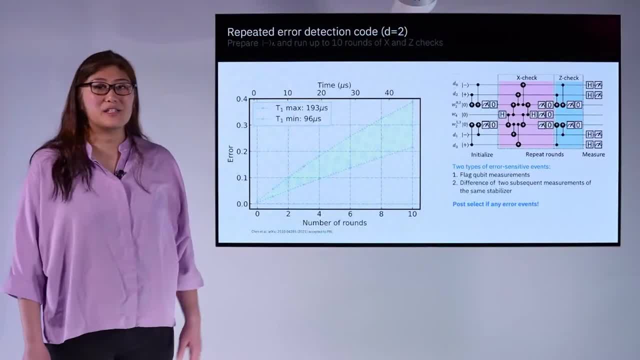 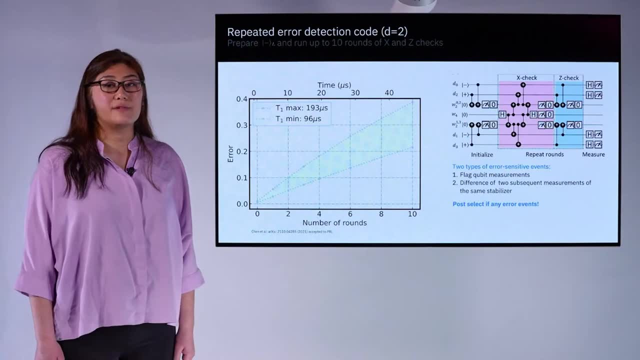 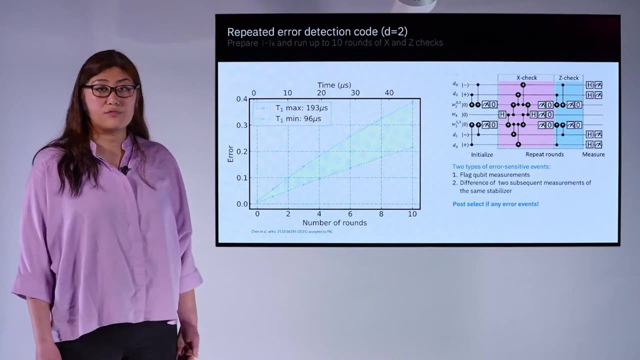 which is shown in yellow region in the plot. And longer you try keeping the qubit in one state, it is more likely for the qubit to experience the bit flip error. Now the distance to 412 code encodes one logical qubit into four physical qubits. 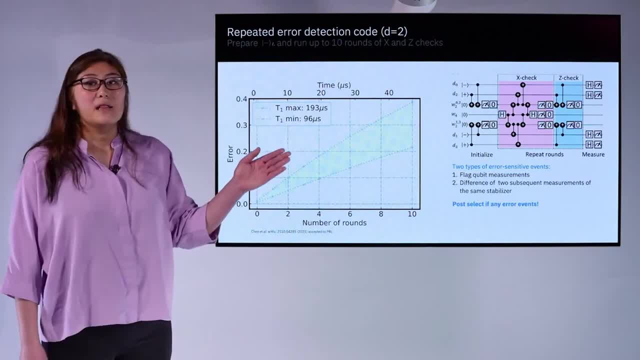 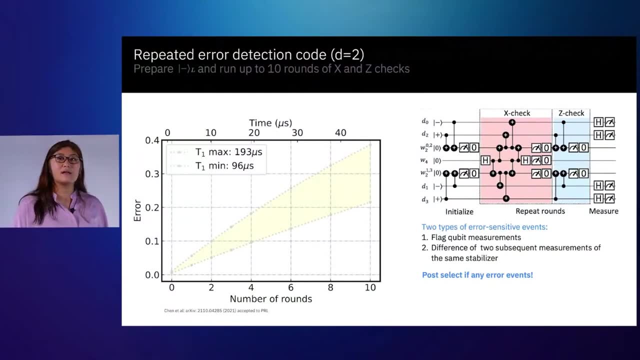 and, as you see in the circuit here, the first part is how we encode the qubit, and pink part of the circuit is how you detect phase errors and finally blue checks for bit flip errors After initializing the state. you repeat this pink and blue block n times. 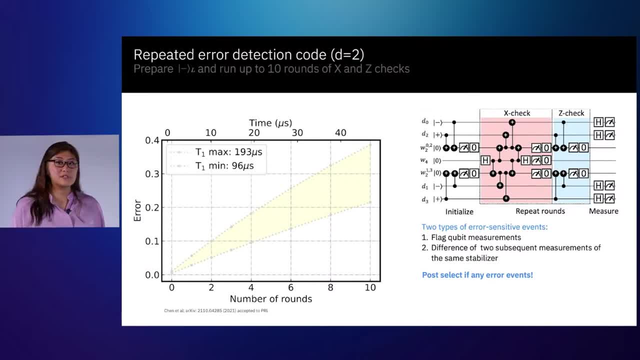 that's the number of round you see in the x-axis to the left. and then you repeat this number of round you see in the x-axis to the left and finally, measuring the data qubits to see if the state of your measurement at the end. 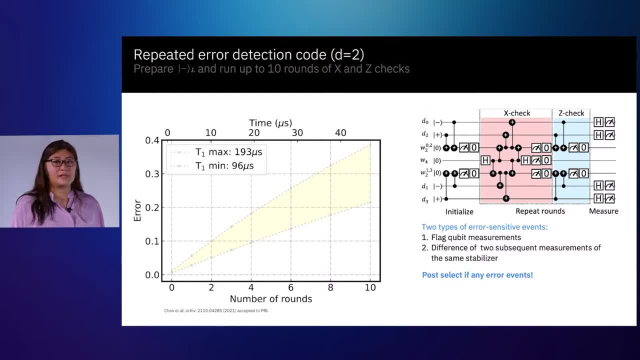 is the same logical state as what you have prepared. So in this circuit there are two types of error-sensitive events: One, when there is an error on flag qubits and second, when the two subsequent measurements of the same stabilizer are different. 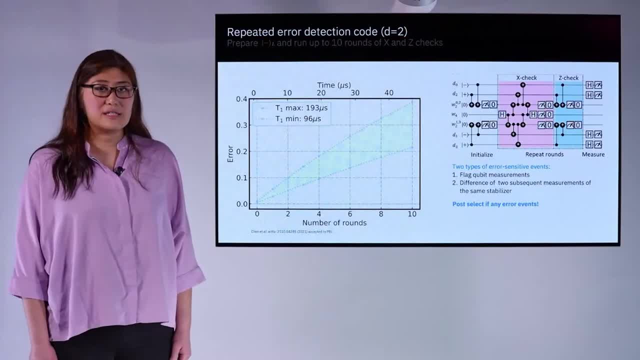 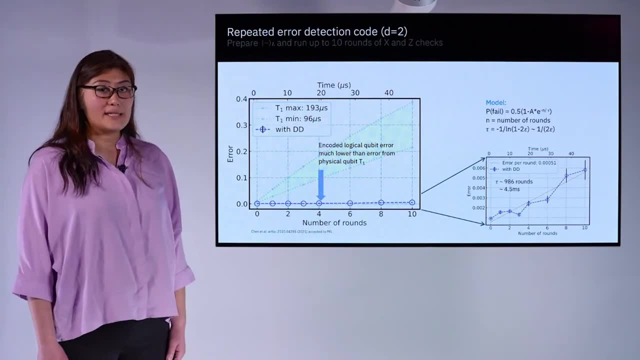 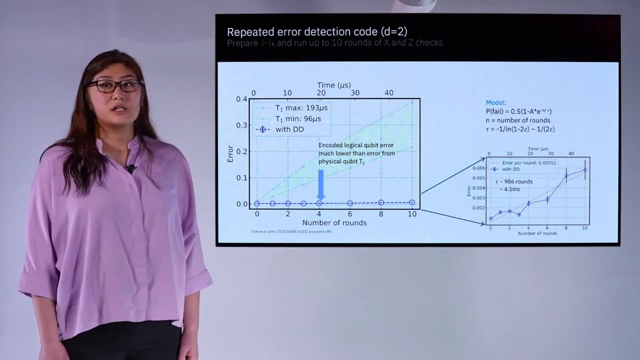 and we post-select if there's any error event. Here in blue I am plotting error after preparing a logical minus state and running the error detection circuit n times. As you see, encoding logical qubit error is much lower than the error from physical qubit T1,. 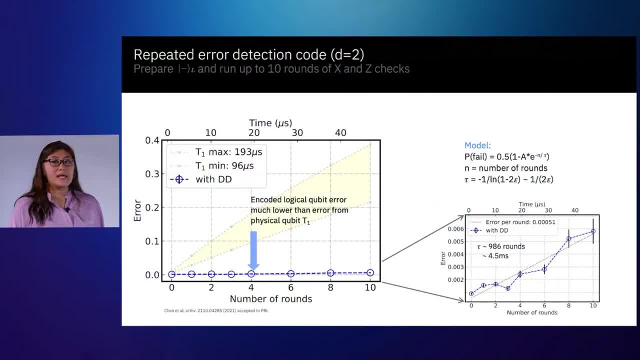 and when you zoom in and fit to a model, we can obtain lifetime tau which is around 986 rounds, and this corresponds to about 4.5 milliseconds from converting to unit of time, much, much longer than physical T1 times. 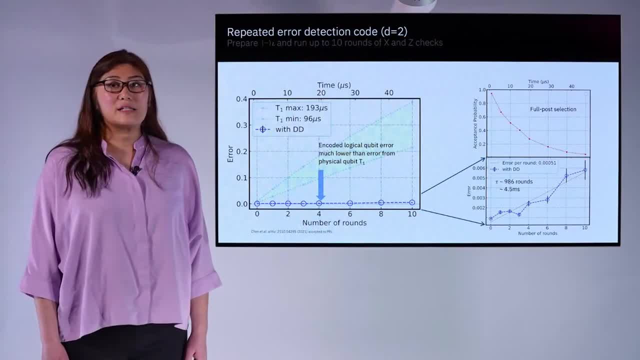 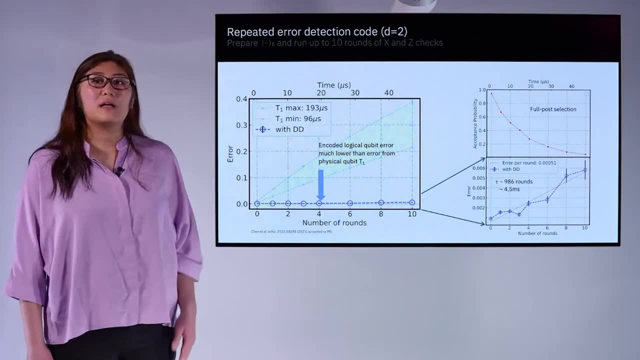 Finally, what we need to note is that, since this is an error detection code, we are throwing out data when we detect an error. As you see in this acceptance probability plot in red, as you run more and more rounds, there are less and less accepted results. 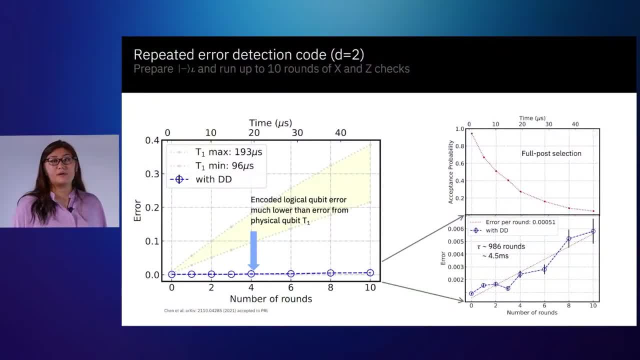 throwing out more and more data. In our recent paper, Calibrated Decoders for Experimental Quantum Error Corrections, which has been accepted to PRL, we evaluate a new decoding technique and consider partial post-selection that will allow us to keep more data than doing full post-selection. 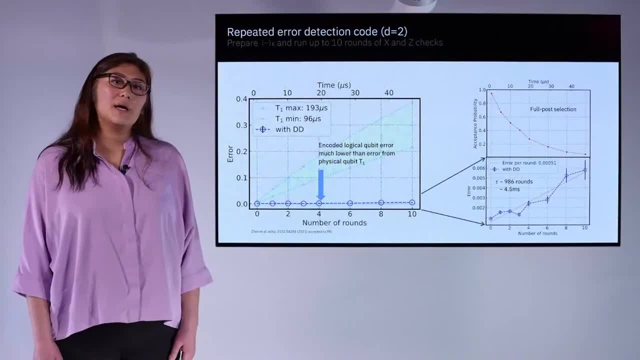 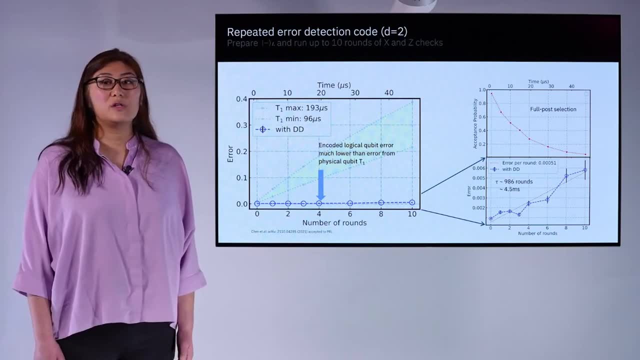 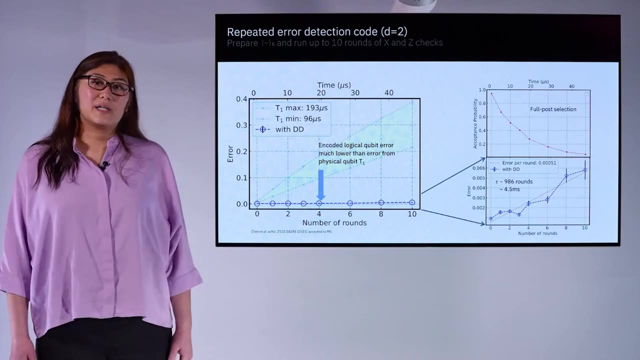 as shown in the example here. But if you really want to have a scalable error correction code, you need at least distance 3, total of 23 qubits in a heavy hexagon lattice to correct an arbitrary error. And that is the next experimental demonstration. 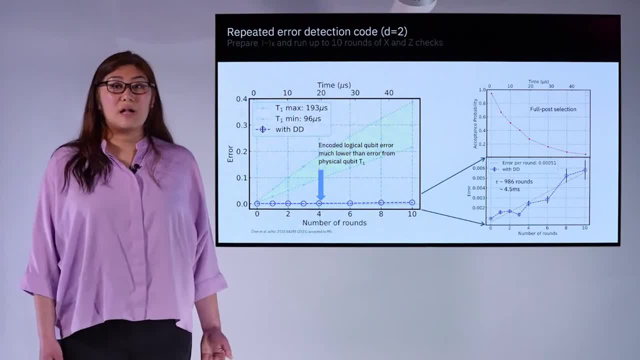 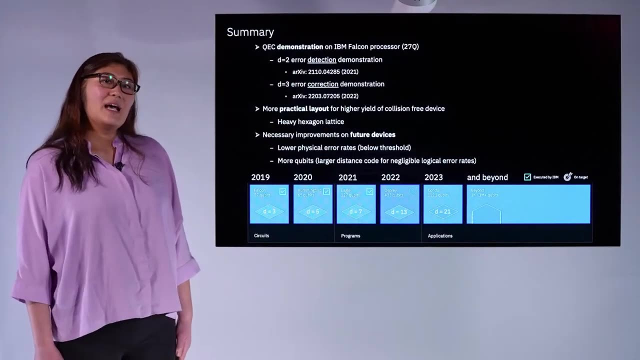 Which can also be implemented on a Falcon processor, in our new paper, Matching and Maximum Likelihood Decoding of a Multi-Round Subsystem- Quantum Error Correction Experiment. So here's the summary of what we talked about today. I just showed you: D equals 2. quantum error detection demonstration. 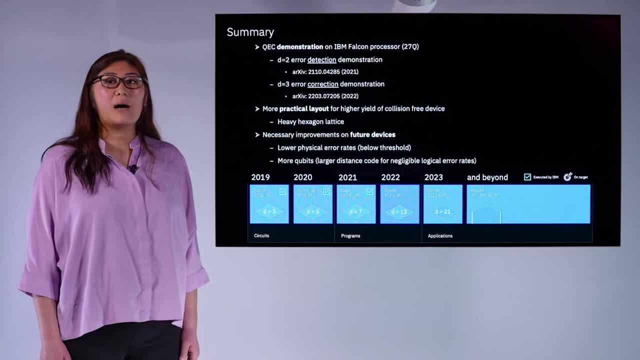 on IBM Falcon processor where we saw a benefit of logical encoding. Using the same device we can map a D equals 2 quantum error detection in a heavy hexagon lattice which provides more practical layout with higher yield of collision-free device And jumping to the very bottom of the slide. 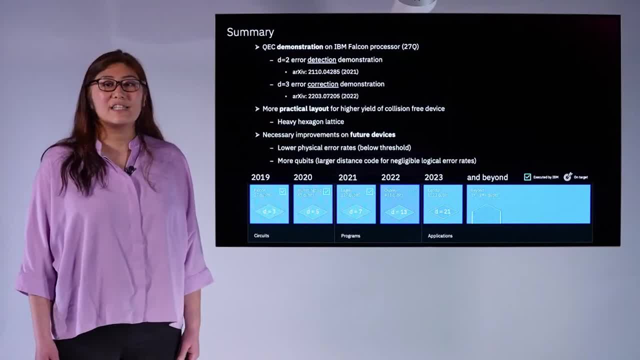 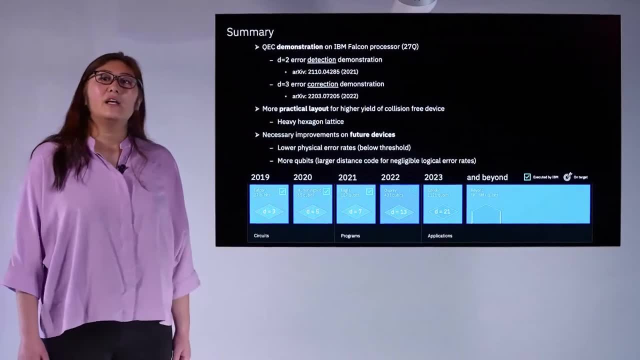 you can see IBM's current progress on the hardware roadmap. We are on track to our target systems And note that as the number of qubits increases, we can see that the number of qubits increases and the number of qubits decreases. 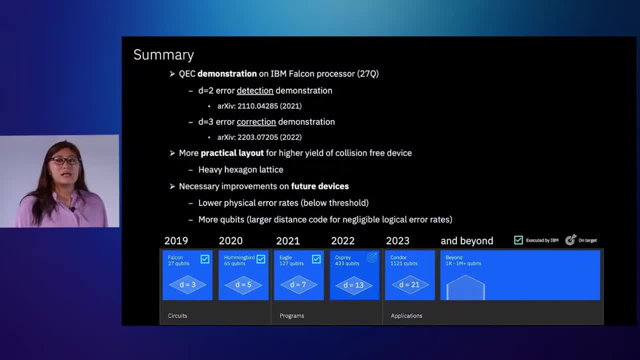 and the number of qubits decreases and the number of qubits increases and the number of qubits increases in each generation. you can map a larger distance code. So as we increase the number of qubits, we need to work on lowering physical error rates. 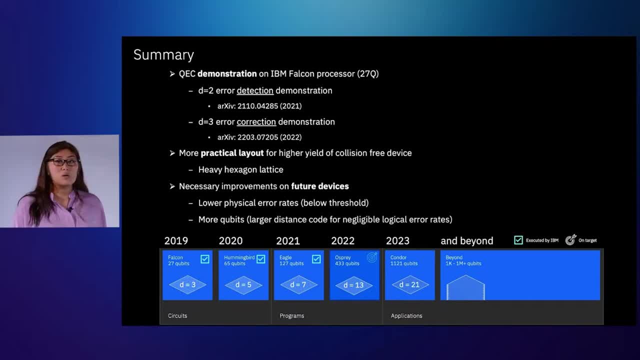 bringing them to well below the threshold. so as we encode a logical qubit into a larger number of qubits, we can achieve negligible logical error rates that we can use to solving more complex problems. Thank you for your attention, Micah. thank you. 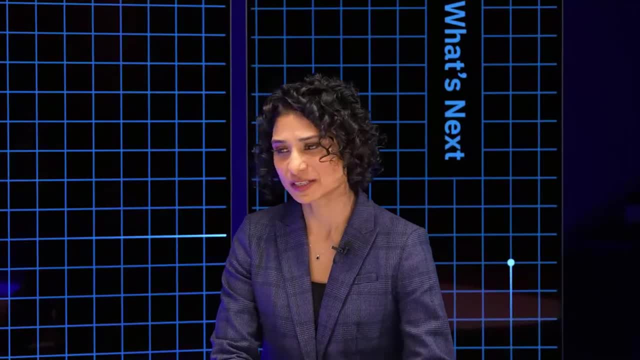 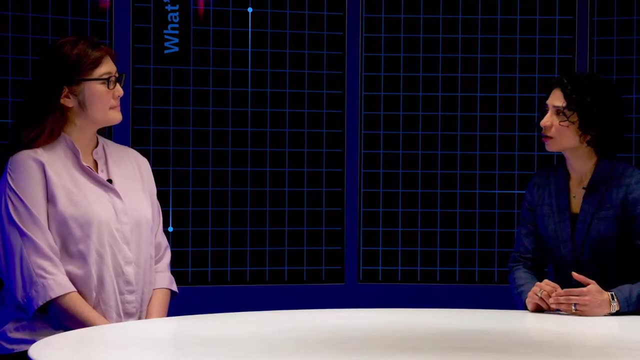 I have questions for you that run the gamut from very detailed to big picture, So get ready To start out with. when you were talking about the change in hardware structure, you mentioned that the newer structure results in fewer collisions. Could you talk with us about frequency collisions and what that means? 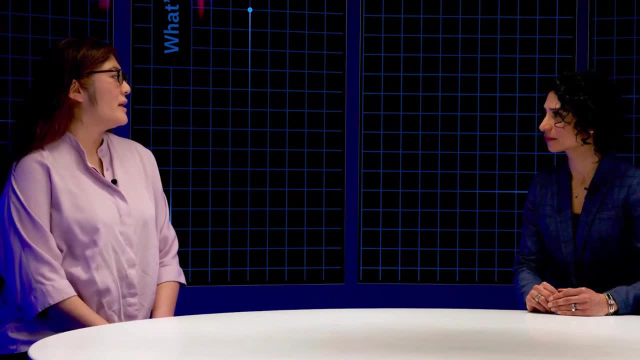 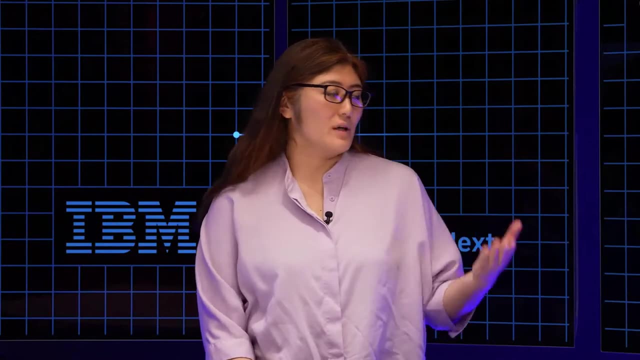 Yeah, So at IBM we've been working with fixed frequency transmon qubits. So that means that we have a fixed frequency qubit, that we don't modify the frequencies of the qubits and we always have an always-on coupling. between the neighboring qubits. So say, if the two qubits are coupled, when both qubits have the same frequency, that could be a problem. So say, in controlling one of them it could actually couple to the second qubit. And also in transmon qubits. there's not only this 0, 1 state that we use for qubits state, but there are also higher transitions that you have to worry about. So there are a lot of not just a 0, 1 frequency. 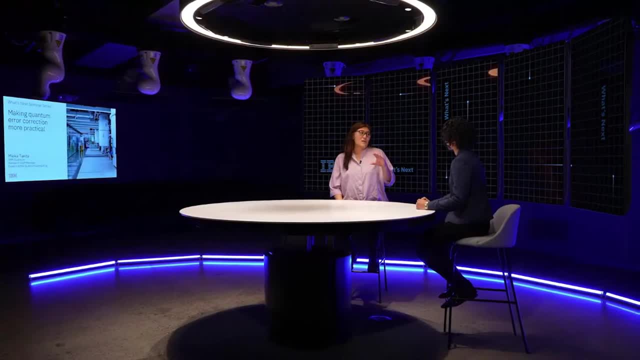 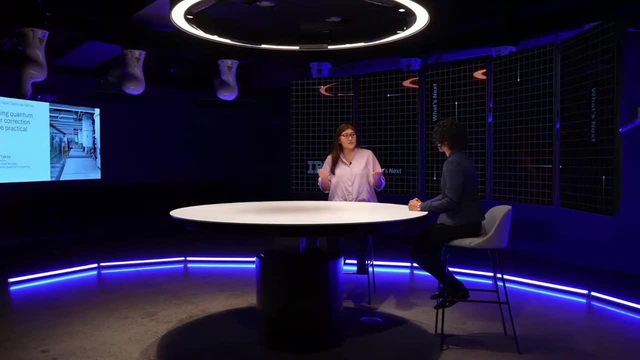 but there are a lot of other frequencies to the specific qubit that you want to avoid having coupled to. So by changing the lattice from the square lattice to heavy hexagon lattice, each qubit is coupled to less qubits. So by having less qubits neighboring them, you have less chance of having a collision, So that actually leads to having better yield and fabricating a good collision-free device. So it's not that qubits are colliding less frequently, rather that the frequency collides and the collisions are happening less often. 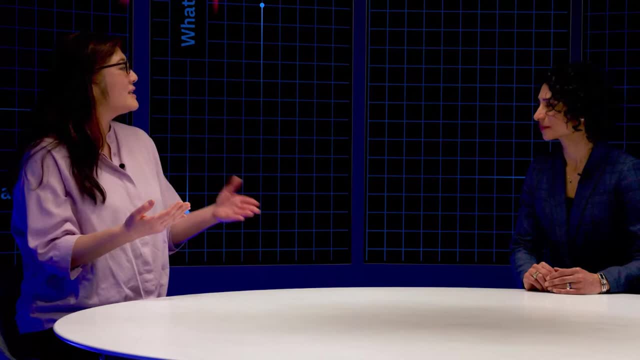 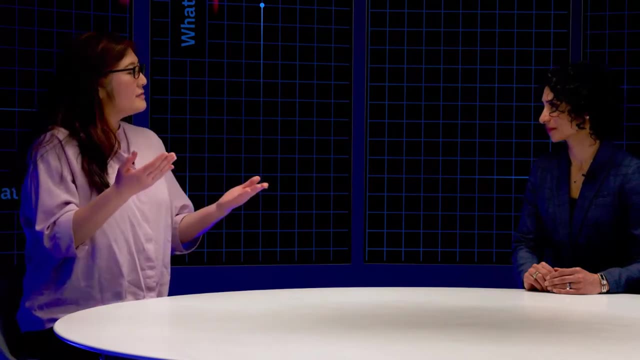 Right, So it's from the beginning. Once you make a device, the qubit frequency. we don't change it, So it's a defined parameter. So once you make the device, if there's a collision you can't really use that. So then you have to try making a new device with different frequencies and you want to make it so that there are no collisions. Got it? Thank you for the clarification. You also mentioned that the newer Falcon devices have achieved higher coherence than the older ones. 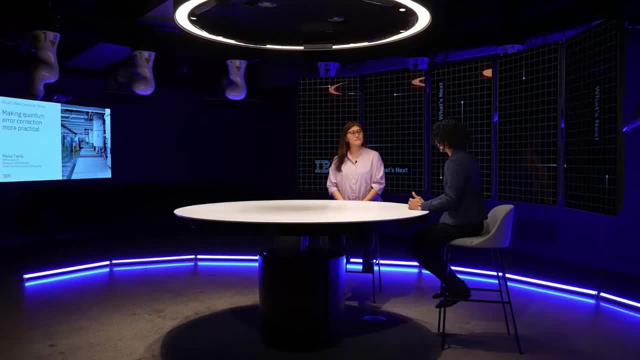 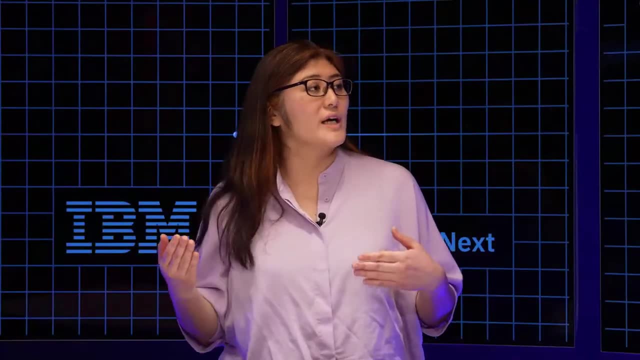 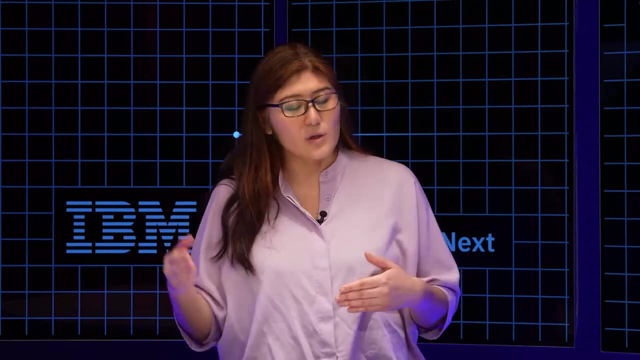 What relationship does that have to the error correction demos that you're working on? Yeah, it's a great question. So, with higher coherence, it also relates to lowering the physical qubit error rates. So I mentioned about how, with the quantum error correction demonstration. 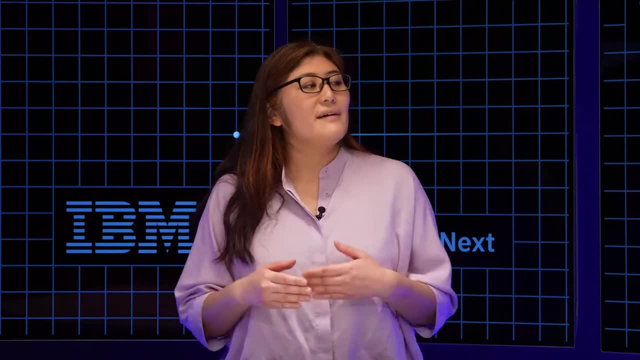 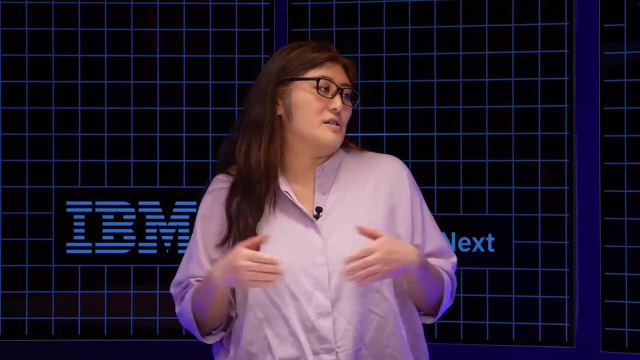 we want to have lower and lower physical errors, So by having a long coherence you could achieve lower error rates. And also there are times that the qubits are just going to be idling, And just by having that longer coherence. 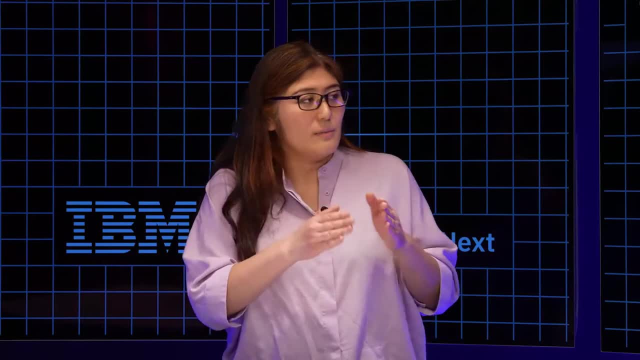 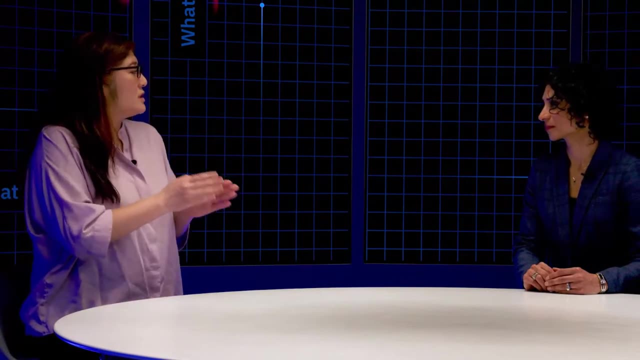 you don't have to have the gates as fast as you can. If you have the gates with the same length, if you have a twice as long coherence, the error that's going to accumulate during that same period of time is going to be less. 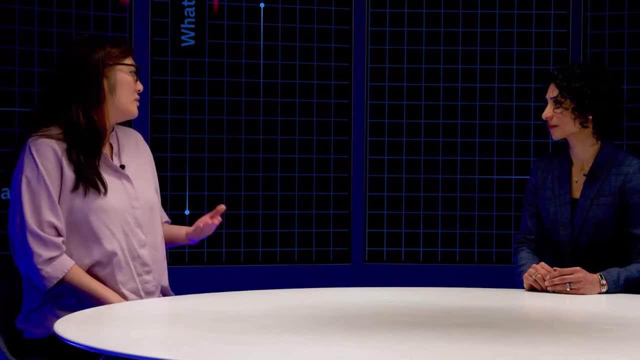 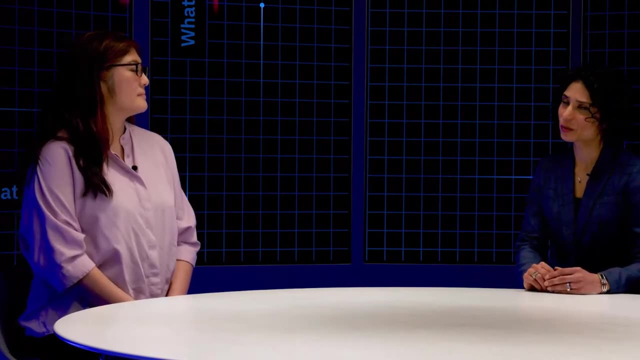 So that is going to directly translate into how the logical qubit performance will be. So the coherence is another really important factor. Yes, Got it. So when we think about what's in the wings, what are the next steps towards improving? 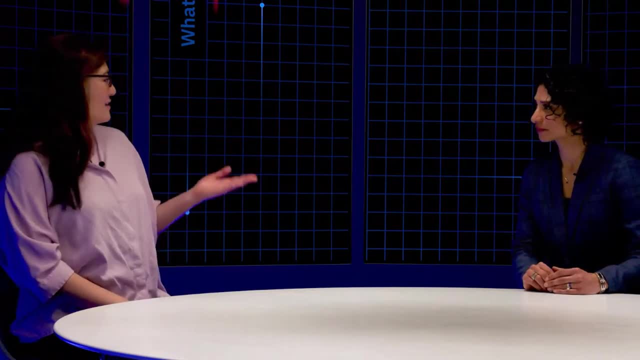 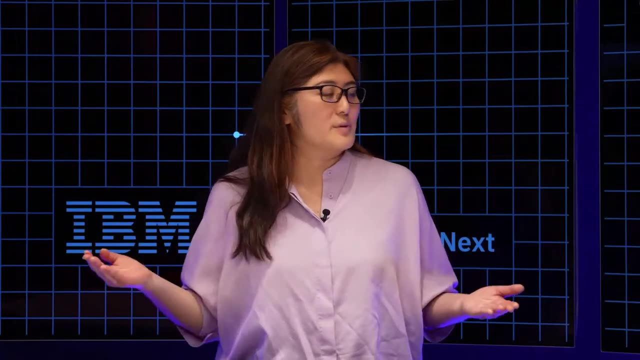 logical qubit performance. Yeah, So you know again the physical error rate that has to go down. we also want to improve the measurement capabilities- Right now the measurements are pretty long- And also in our systems and superconducting qubits. 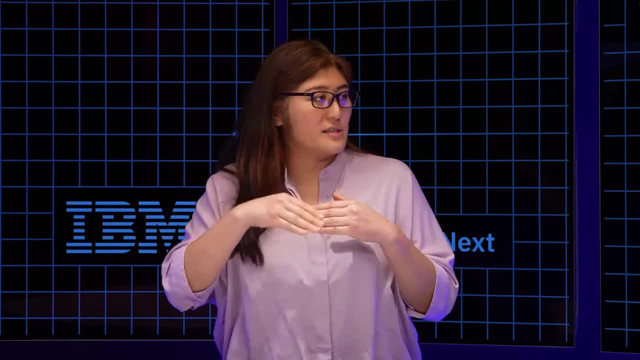 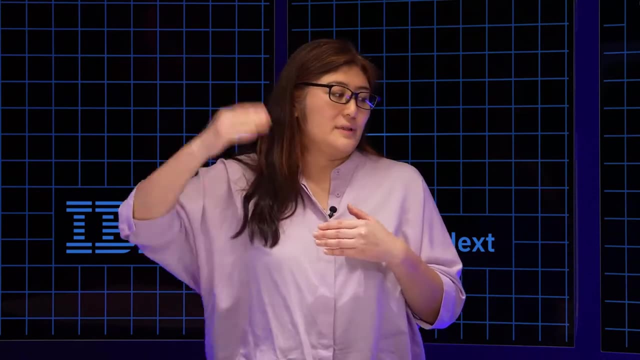 as I mentioned about higher states, that's not just a zero-one state in just one qubit, but you do have some leaked states that could be there. So we want those errors to go away. So we need to reduce a lot of errors. 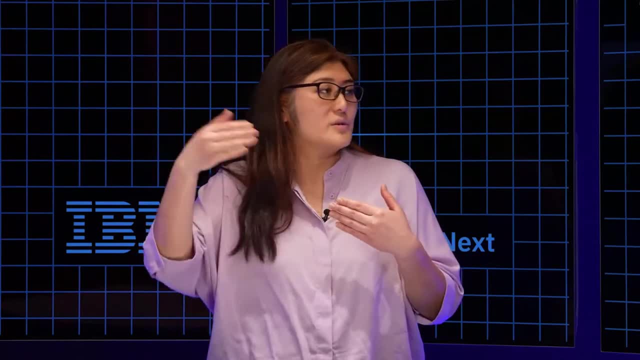 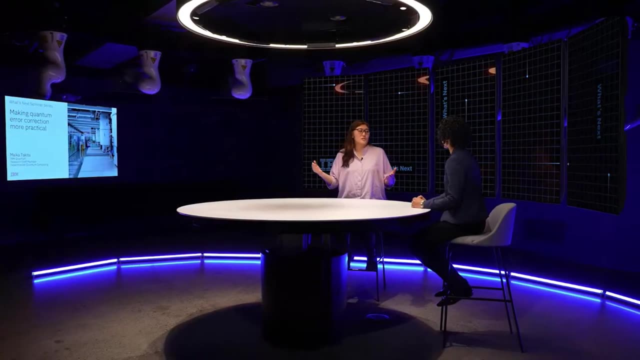 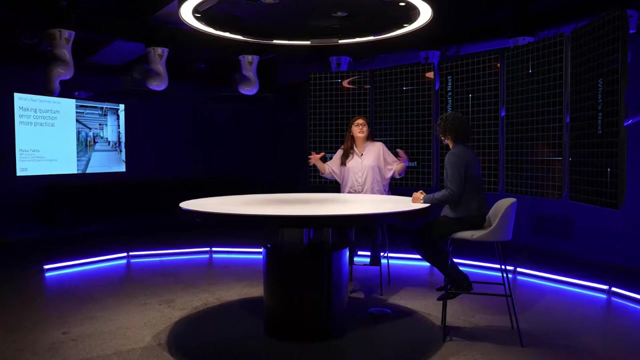 not just the gate errors, but also measurement errors and those leakage errors, But also, as you grow, the larger lattice, you could try to implement these new logical qubits. But also, we do want to think, not just making larger and larger devices. 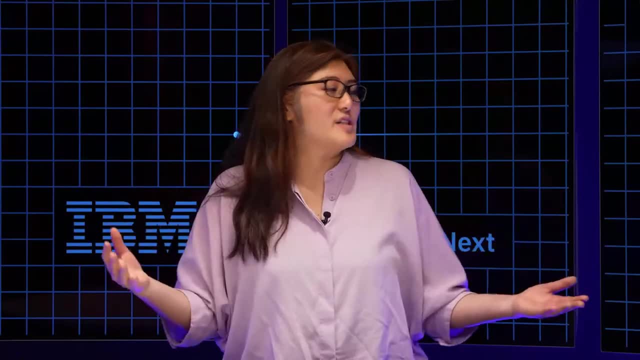 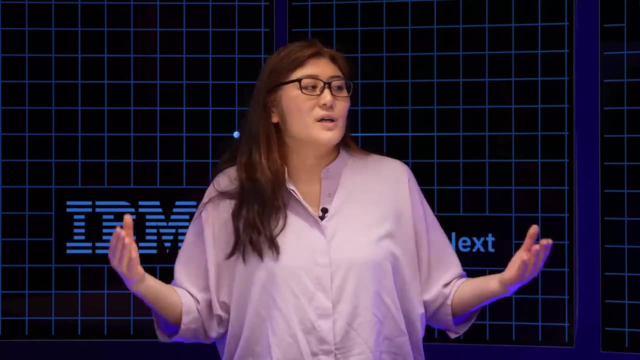 but we also want to come up with a way to have a more efficient error correction. And a theory aside, there's a lot of progress that's been made- that's not just in the planar code, So we also want to start considering. 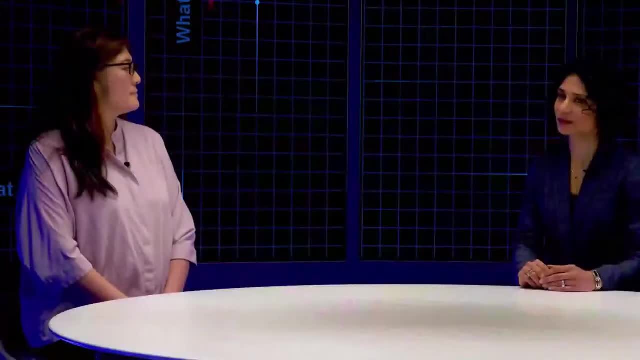 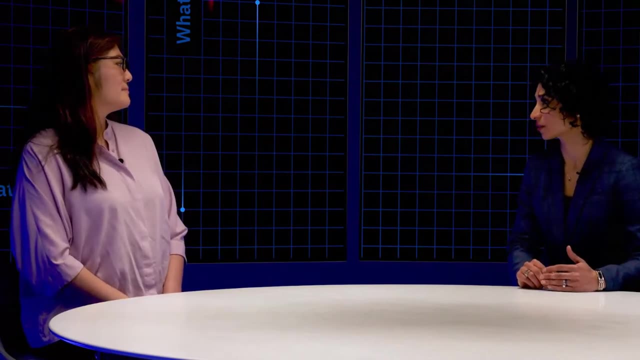 how this could be done in a hardware. Got it? So let's jump it up. It sounds like error correction is something that we all take for granted in classical computing, but it's a reality and an important problem to be solved. Would you say that quantum error correction 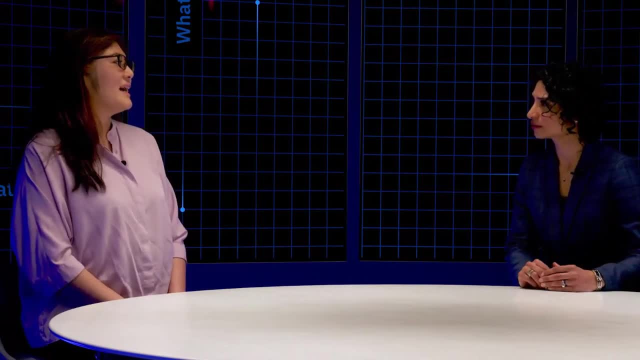 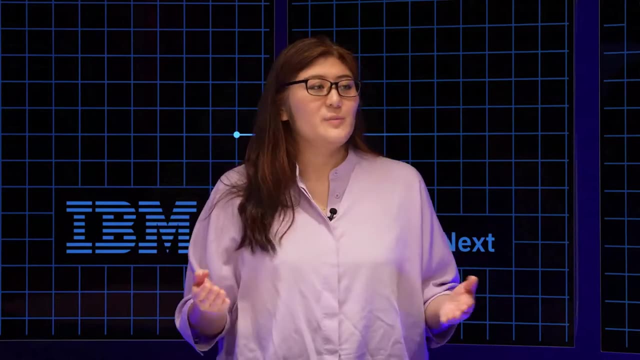 is critical to the future of quantum computing. Yeah, absolutely So. quantum error correction by having that ability to correct for some errors. you know qubits are quantum systems are always going to be noisy, So we need some way to correct for those errors. 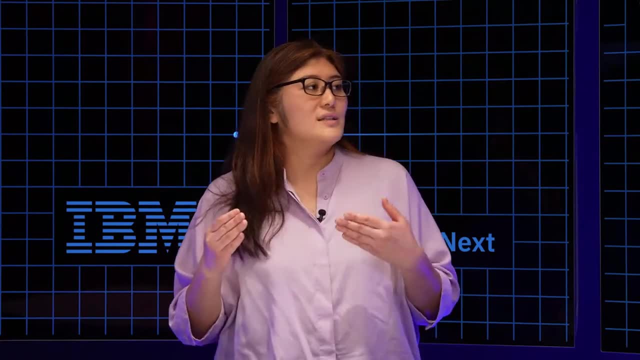 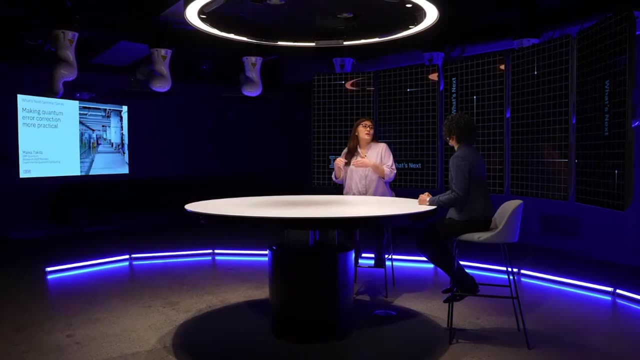 especially if you want something accurate. Also, if you want in theory, if there are, if you have a quantum computer, say, then that definitely could give you an advantage, say an exponential advantage. That doesn't necessarily mean that. 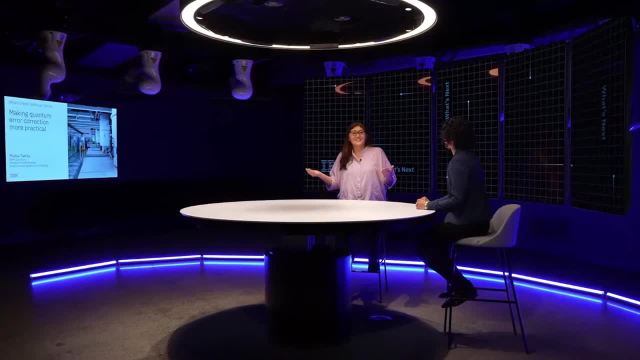 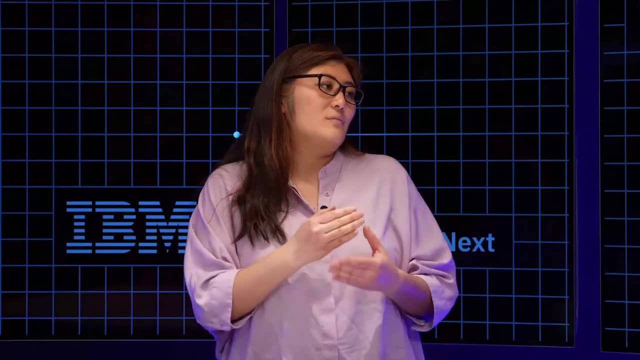 you know, without error correction you can't do anything right. But you know, with the proof that we have now within theory you do need error correction for these really complex problems. But even without there are a lot of things. 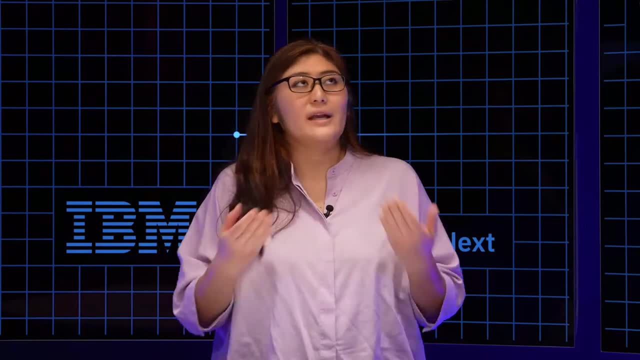 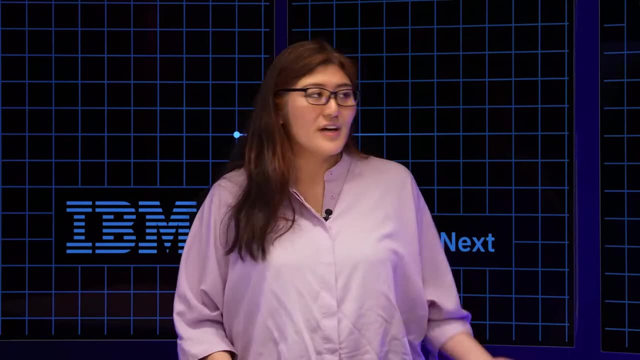 that you might be able to try in the near term. where you know, we now have a device that is over 100 qubits- 127 qubit- Eagle device was just deployed last year And it's very exciting. It's something that